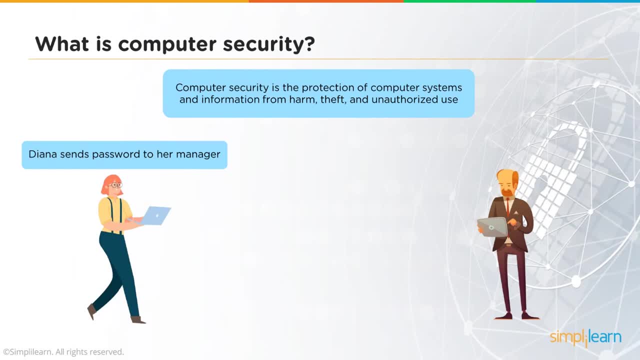 or internal hackers. So in this scenario, Diana is trying to send information to her manager, but the information is intercepted by the hacker and the hacker gets their hand on some sensitive information that Diana is trying to send Here. in this case, it's a password. Now, since the hacker has the password to Diana's laptop, the hacker can. 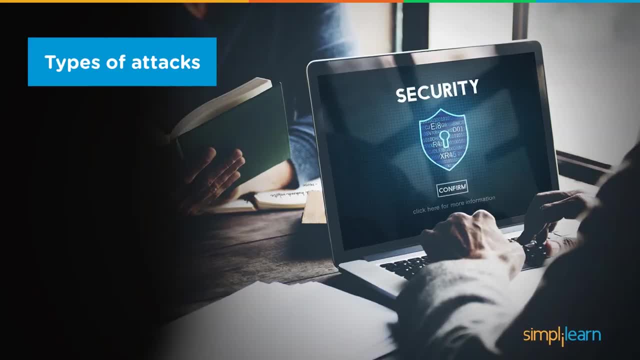 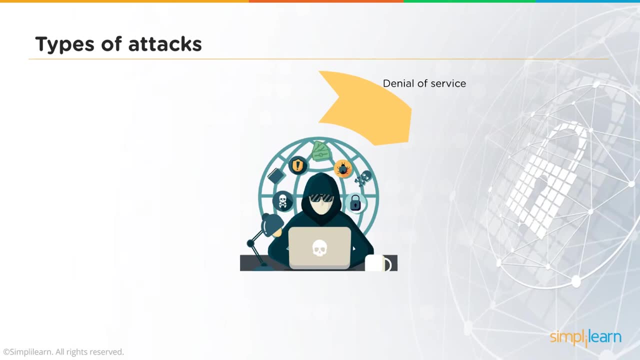 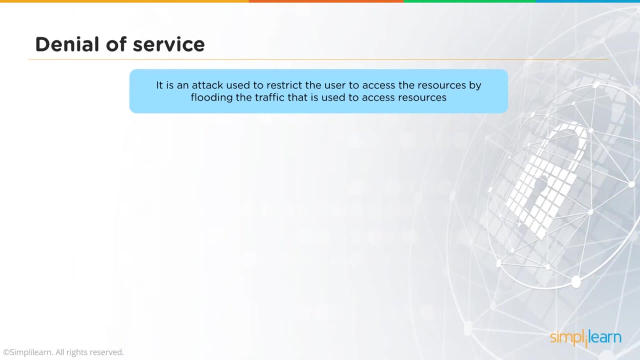 then try to get access and then steal data from Diana. Let's look at the type of attacks on information security or computers. The first one is a denial of service or a DOS attack. In a DOS attack, the attacker normally tries to consume the bandwidth or the resources that are available for 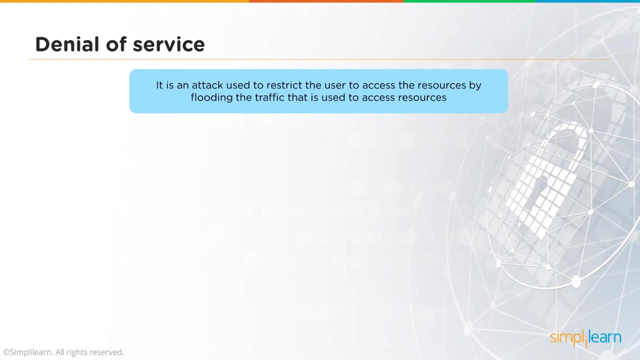 the server that is deploying the application or that is allowing those resources to be given out to the users, And once the hacker has restricted those resources or has consumed those resources, there wouldn't be any sufficient resources for end users or legitimate users to consume. thus, 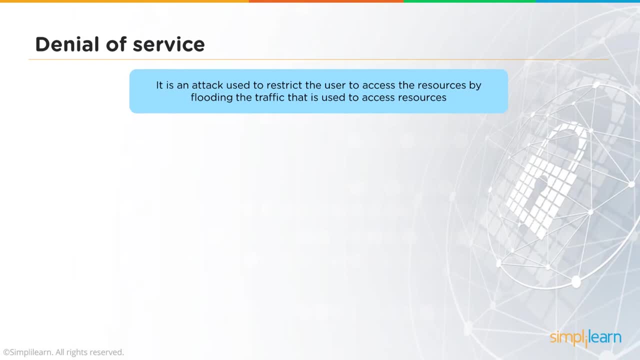 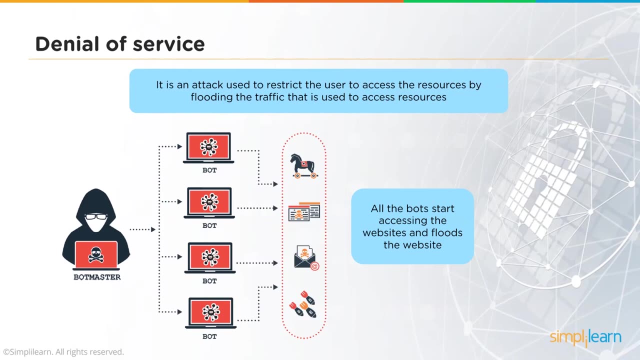 denying them the legitimate service and hence being called a denial of service attack. Here, in this case, there is a bot master. There are various bots, And these bots would then generate traffic or malwares and then try to attack the victims. A bot is. 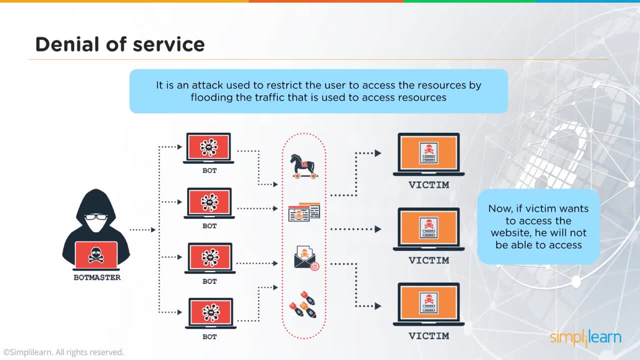 nothing but a software that can be installed on a victim's machine, using which the attacker can then remotely send commands to the bot, and the bot will then create that traffic to attack the victim. So here, in this case, the bot is nothing but that software that has been installed on the victim's. 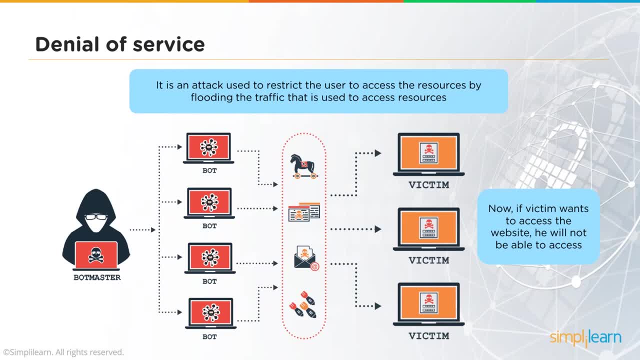 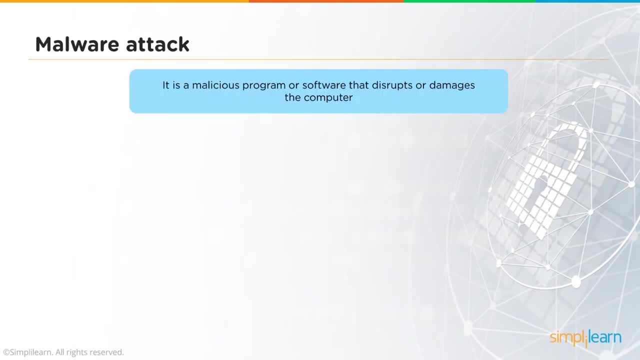 machine that allows the bot master- or the hacker in this case- to remotely send commands to the bot to do appropriate actions. The next attack we are going to talk about is malwares. Malwares are nothing but malicious softwares that pose as legitimate softwares but will have a virus, trojan or a worm embedded within it. 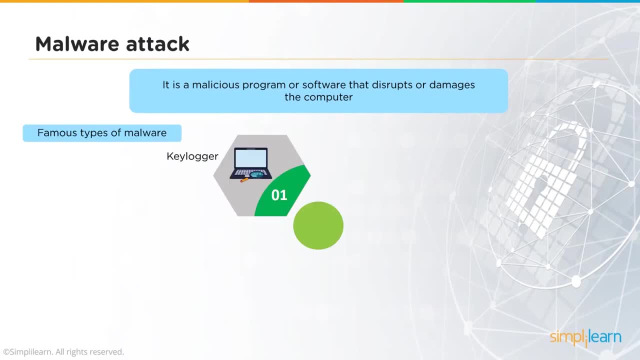 Right, It could also be a keylogger. A keylogger is nothing but another software that is created to catch all the keystrokes that the user is making, create a copy of it and store it and send it back to the hacker. So, whatever the user is typing, it will now be known to the hacker. 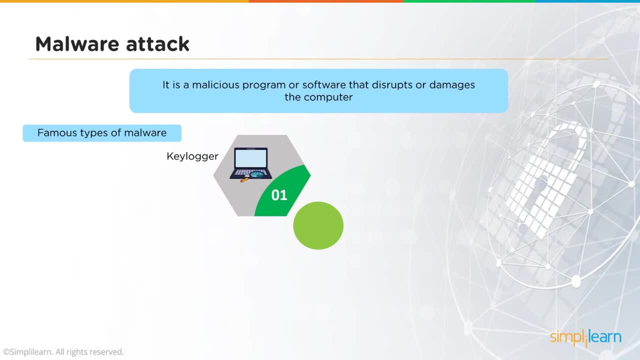 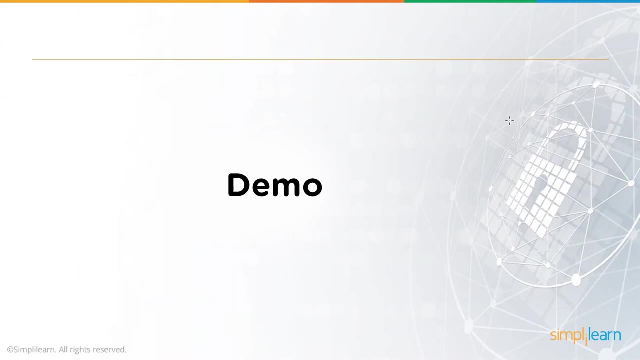 It could be bank details, Passwords, Any personal information that the user might want to keep secret. We are going to look at three different demos here. This demo is just to showcase a couple of things. We are going to look at a keylogger- how a keylogger works this virtual machine here. 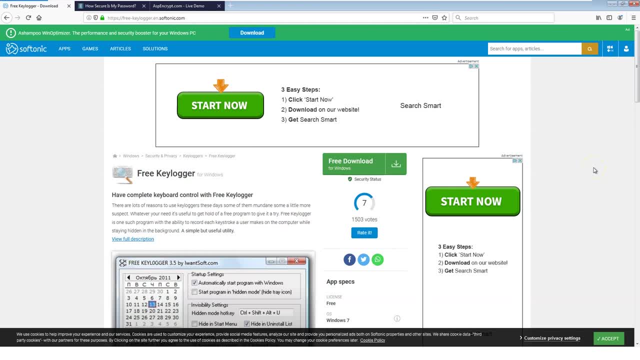 And I've already downloaded a keylogger and installed it. The idea of this demo is to showcase how a keylogger functions Right, So you can see online on the screen. we are using a freekeyloggerensoftanicom. We are on this site. 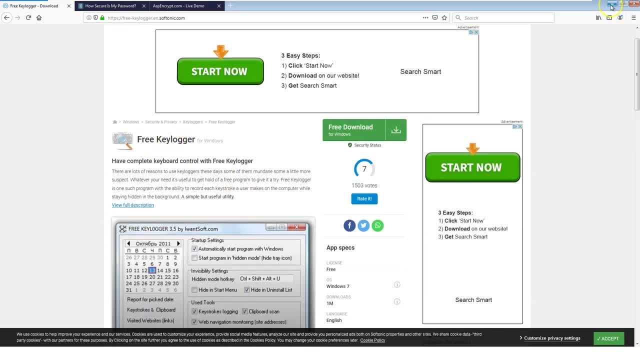 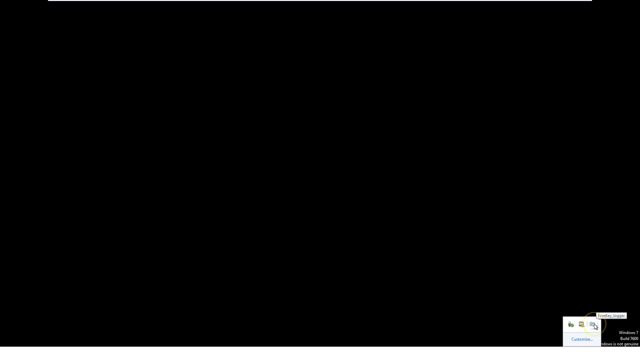 And you can download the freekeyloggerensoftanicom. So we are going to download the free keylogger right from here. What I've done using my demos is that I've always have a keylogger running in the background to capture all the keystrokes that I've been doing whenever I'm doing any demos. 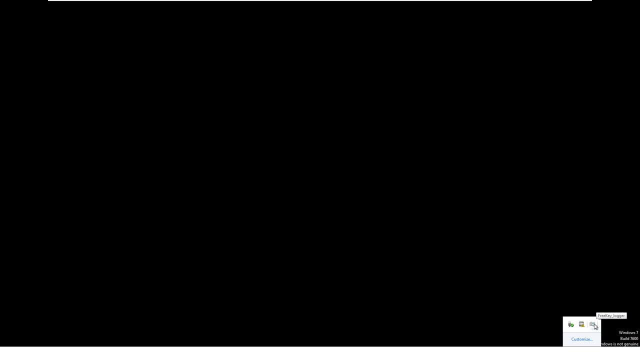 So this keylogger here can actually be hidden in the taskbar, But for our demo purposes I've kept it visible. When you click on it, it will open up and give you a basic screen where you can start navigating about the keylogger. 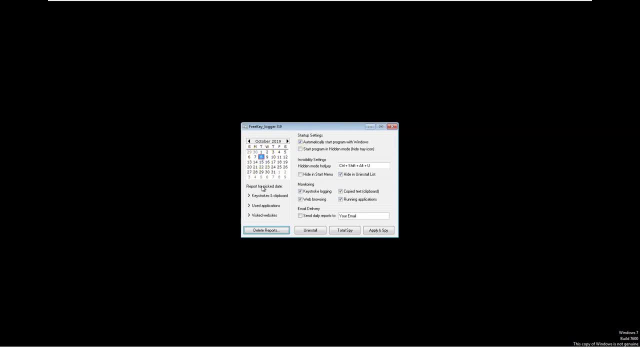 Now you can see that on 8th, which is today, It already shows some keystrokes, Applications And some visited websites, as you can see, already been browsing using the browser over here and which has been recorded by the keylogger in the background. 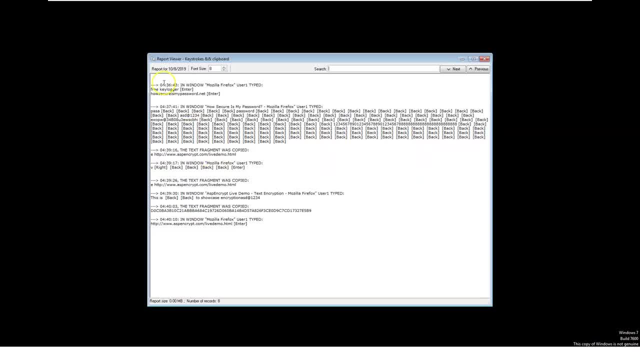 And just to give you an example, if I click on this file, you will see all the keystrokes that I have been doing so far And you can see I've gone to this. I've opened up my Mozilla Firefox. I've typed in a keyword. 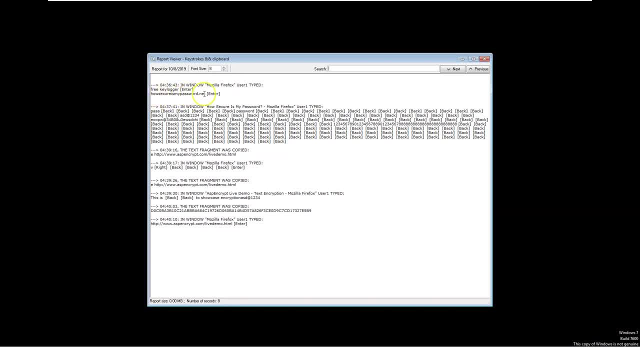 of freekeylogger. Then I've gone on to the website howsecureismypasswordnet, in which I may have tried out a few passwords myself. And then I've gone in, I've copied, pasted this URL into the browser window and you can see. all of this has been. 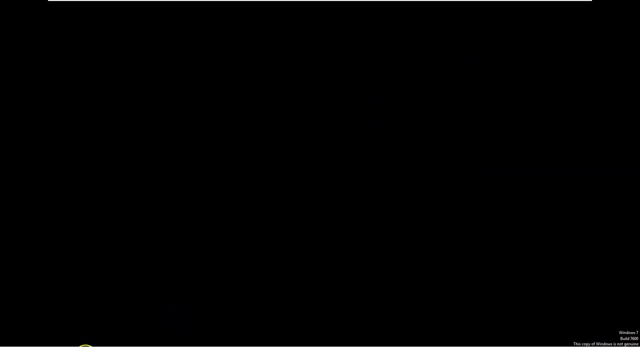 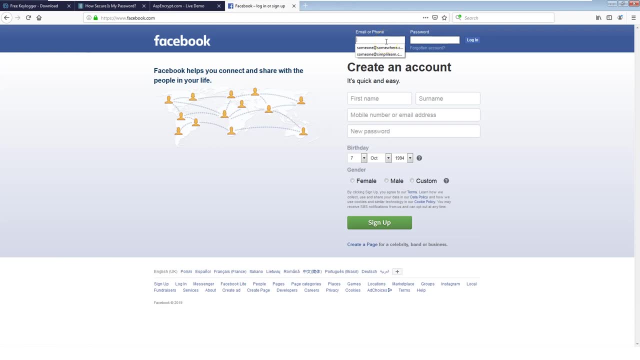 recorded. And just to emphasize on that, let's go on to another website and let's say, let's go to facebookcom. I'm not actually going to log in, I'm just going to type in a random username- So someone at simplylearncom- and a password like ASD, at the rate one, two, three, four. 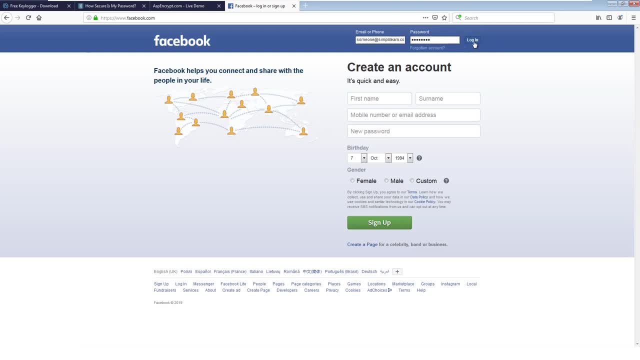 And I'm going to try to log in. Obviously, the login is going to fail because this account doesn't exist, but we want to see what happens in the background when the keylogger picks up the keystrokes that we have typed. So let's open up the keylogger again and go and see what is there in the keystrokes and 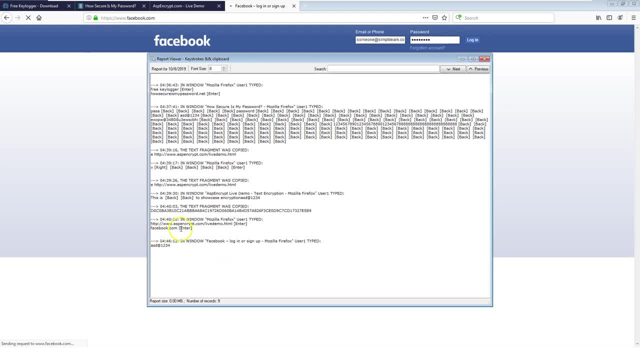 clipboard And you can see over here that we typed in facebookcom enter and then we did not type in the username. That's the difference here. We selected it from a dropdown, So a keystroke logger or keylogger has not been able to capture that input. 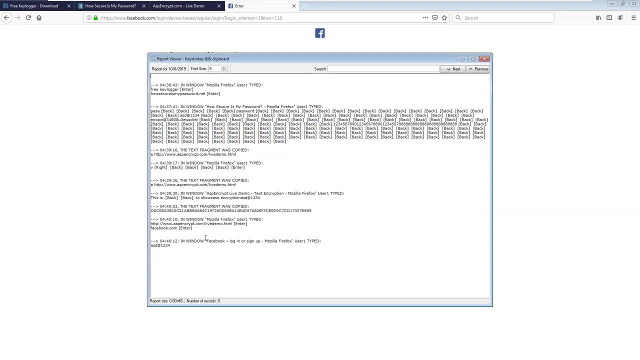 A keylogger, in its essence, is only records. It only records something that has been typed in by the user- real time. Since we did not type in the username, it did not record that username, but we typed in the password and you can see the password over here. ASD at the rate one, two, three. 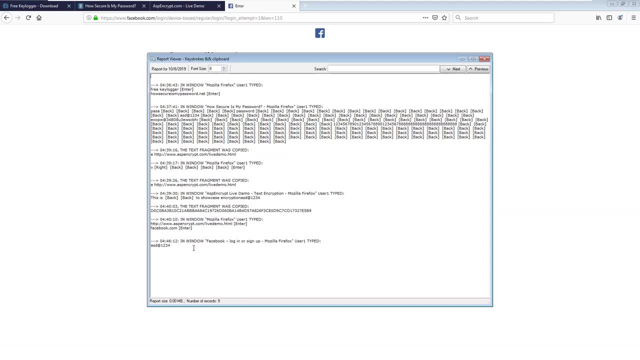 four- And this is how a keylogger works- It only captures the keystrokes that have been typed in real time. So if we use this exercise on our victims and they're just using dropdown menus, at that point in time none of the data is going to be recorded. 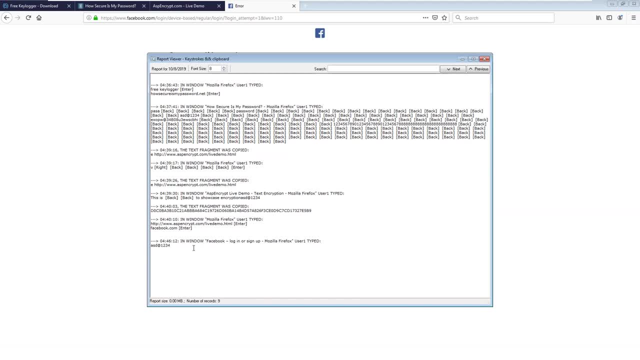 For that activity you would need something which is known as spyware, which would capture, scan and record the keystrokes. So that's the keylogger. You can see the keystrokes on the screen which would capture all of this information. that is going on. 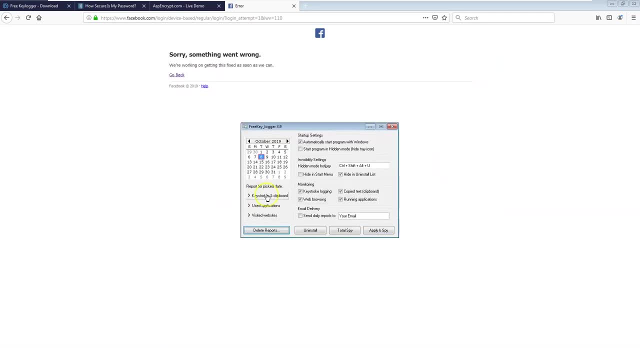 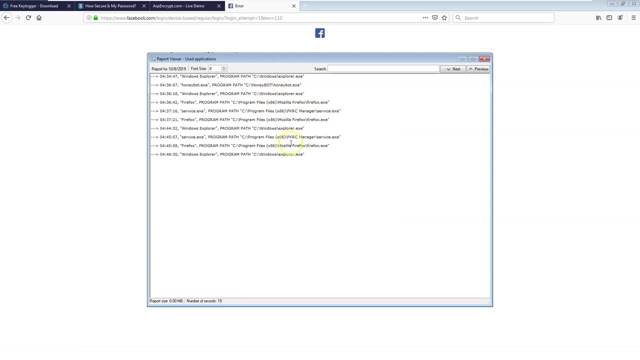 Now, apart from just logging keystrokes, what this software also does is it also has a list of used applications. You can see all the applications that have booted up, along with the operating system, and the ones that have started up after the operating system has booted. 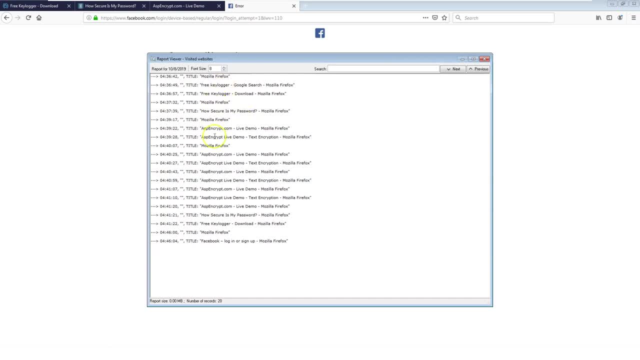 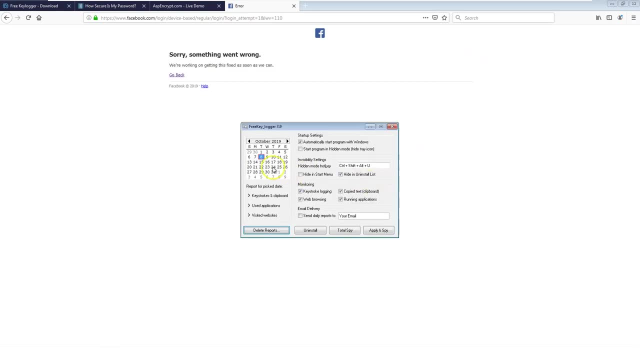 It also has a list of the visited websites. You can see, these are the websites that we have been visiting and they have been listed right here, The last one being Facebook login or sign up. All right, So this can store history for a long time. 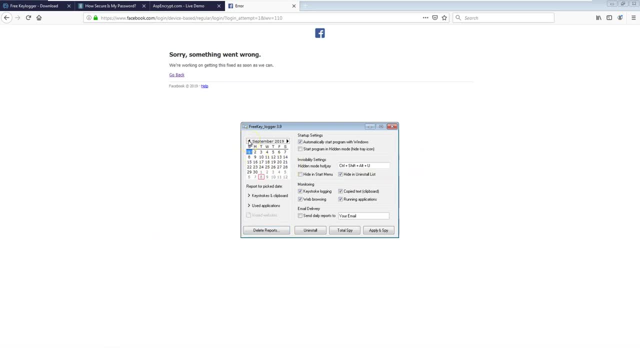 So you can see that this is the list of the websites that we have been visiting, and they have been listed right here, So this can store history for a really long time If I go back in time and if I look at some of the demos that I've been looking at. so 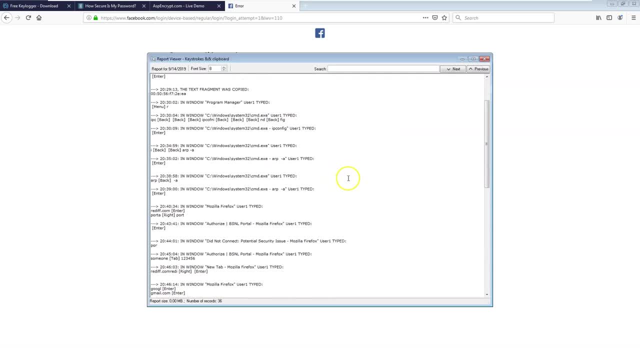 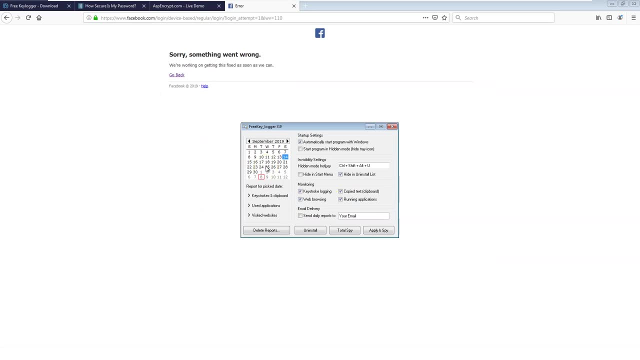 on 14th of September. these were the keystrokes that I utilized when I was doing some trainings or while I was providing some demos on other topics. So a keystroke or a keylogger will store all that information and keep on recording it. 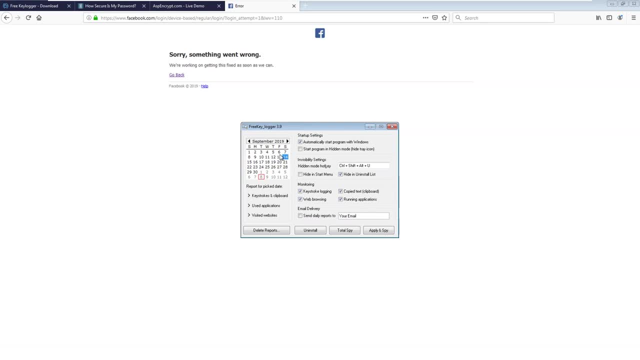 till you actually delete that data or you can reset the keylogger. You can also set up the keylogger to send an email to you as a daily report to a particular email address that you have sent. So as long as it does that, you can use it. 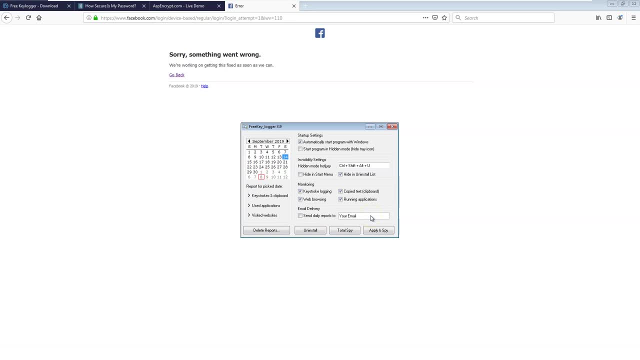 If it detects the internet connectivity. this keylogger will send you an email to the email address that you have specified, with all the keystrokes that it has logged. Now this is the free version. There's again a paid version for it, So you can go and visit this site and see how this keylogger functions. 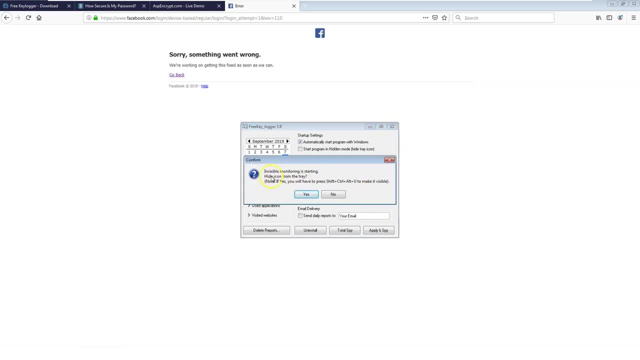 If I press on the X button over here, it will ask me if I want this to be hidden in the system tray. If I click on yes, only using this shortcut will I be able to invoke this screen. So just for demo purposes, I do not want this to be hidden. 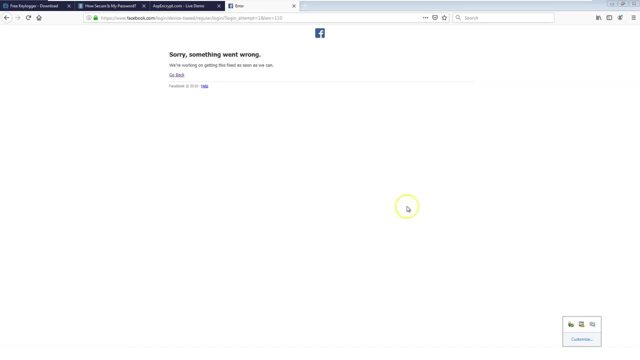 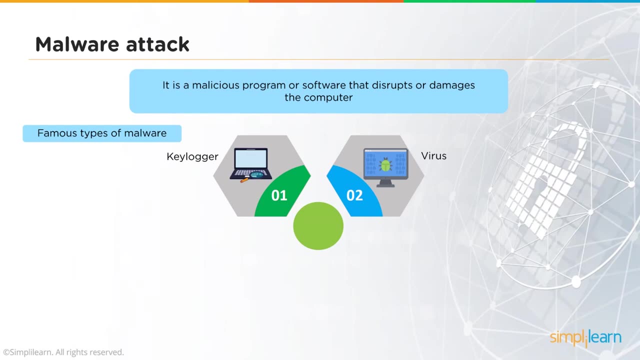 So I'm going to click on no And you can see that the keylogger is still visible over here, So that was the first demo that we are seeing. Viruses, as we all know, are destructive programs that, once executed, would destroy data or harm. 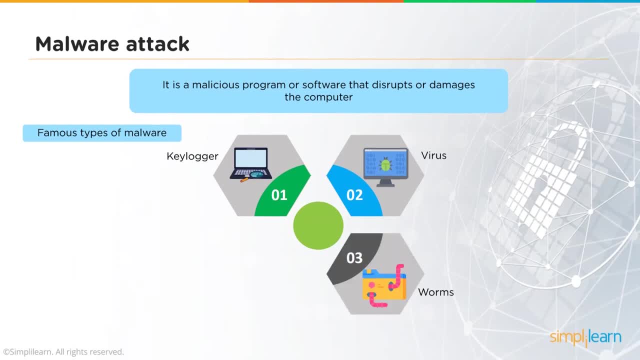 the hard disk or the partition tables. Worms, on the other hand, would be softwares that would be more of a nuisance value, where they're going to replicate themselves in such a way that they would consume the resources of a computer, thus crashing the computer and then requiring a reboot. 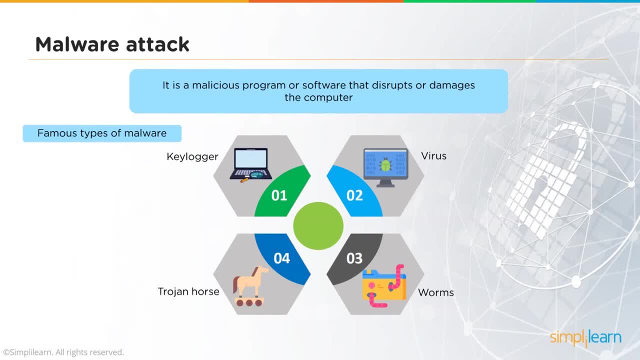 A Trojan horse. This is another software that will allow a backdoor entry or a covert channel to that hacker, where the hacker in this case would then be able to gain access to the victim's machine through the covert channel or the backdoor, without the knowledge and the authorization. 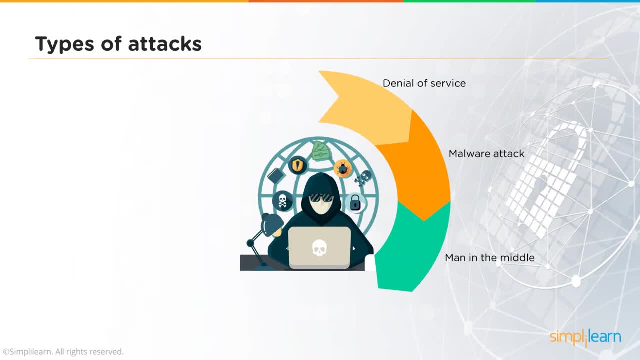 of the user themselves. The next attack: man in the middle. So if you've been looking at the types of attacks that we've been talking about, the denial of service attack was where we are consuming the resources of the system in such a way that they are no longer available for legitimate users. 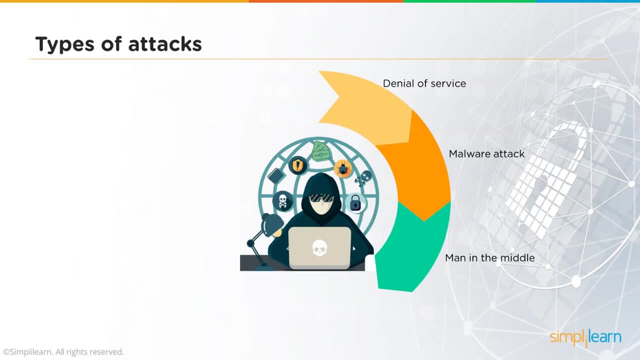 Malwares, on the other hand, would be softwares that would either destroy data or give a backdoor entry to the victim's machines. for the hacker- So a man in the middle attack is nothing but a network based attack, where the hacker is going to try to intercept the communication or the data flow between the victim and the 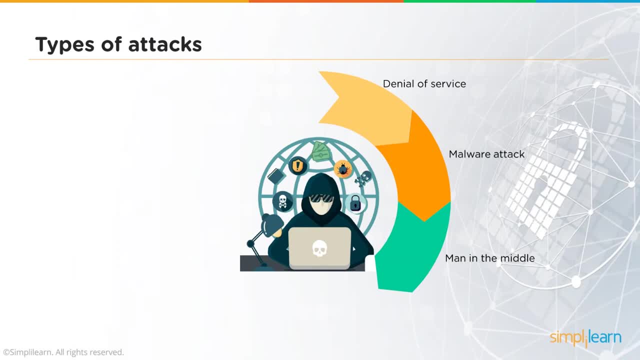 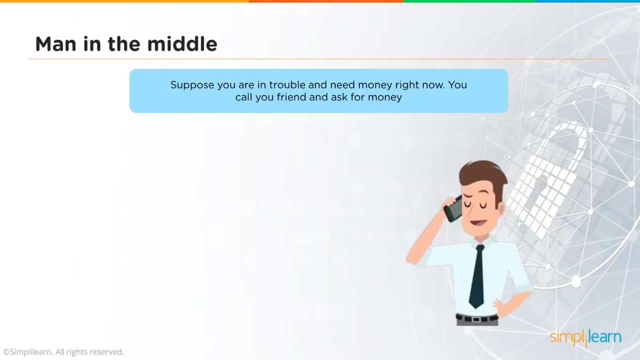 endpoint And thus, when they grab these informations, they would then have captured some data that they wouldn't, they weren't supposed to get in the first place. So here in this example here, suppose you're in trouble And you need money right now and you call your friend and ask for money. 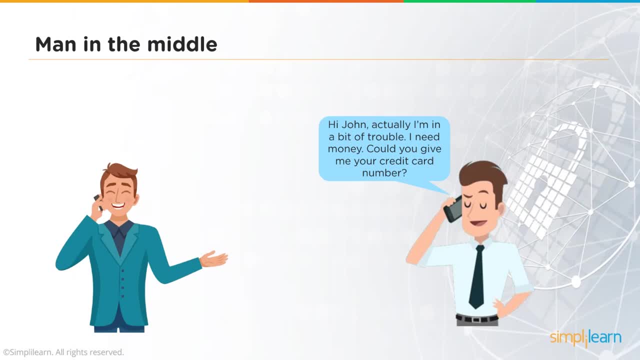 So here the person is calling John, telling John that they're in trouble, and they're asking for John to give their credit card number over the phone. Now this is a legitimate transaction. The friend is actually calling John and asking for some help. 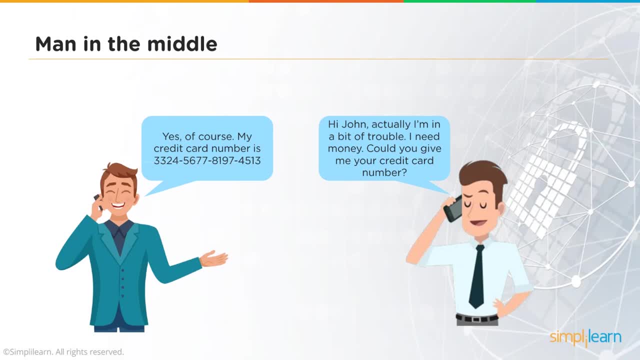 However, when John is providing that help over the phone with the credit card numbers, maybe the CVV number and all of that, and then the OTP at the end of it, at the same time there could be a hacker Doing a man in the middle attack where they could be eavesdropping on whatever is being. 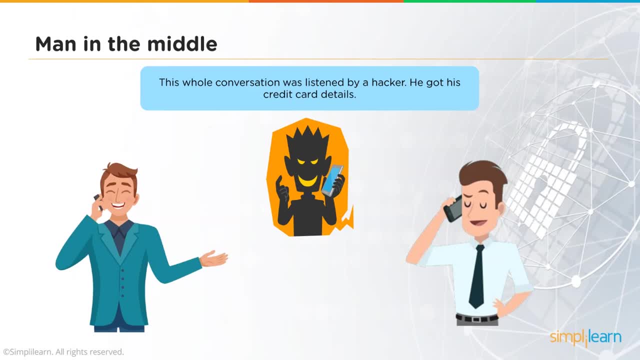 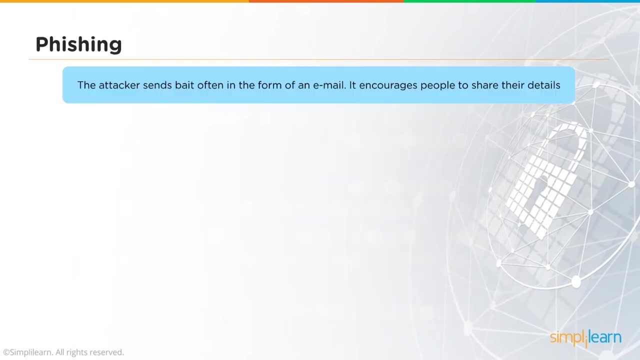 said or whatever, data is being transferred, And once they capture this confidential data, they can then misuse that data to their own gains. The next attack is phishing. Phishing is a very common attack in today's world. It is where the attacker sends a bait, often in the form of an email with a hyperlink in. 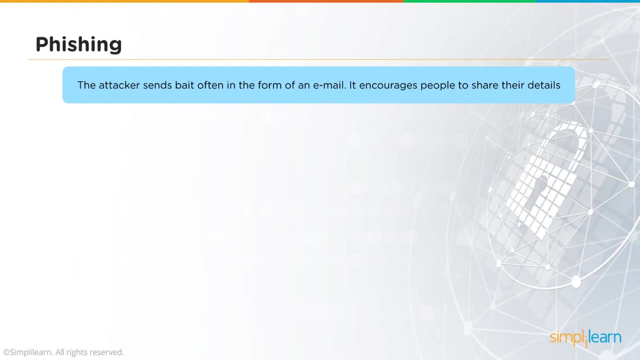 it to encourage people to click on it, thus getting redirected to a malicious server that the hacker is hosting, And then end up Giving out confidential information. Now, obviously, the requirement here is that the email that is being sent out by the attacker needs to look very legitimate and needs to look genuine to the victim for them to go. 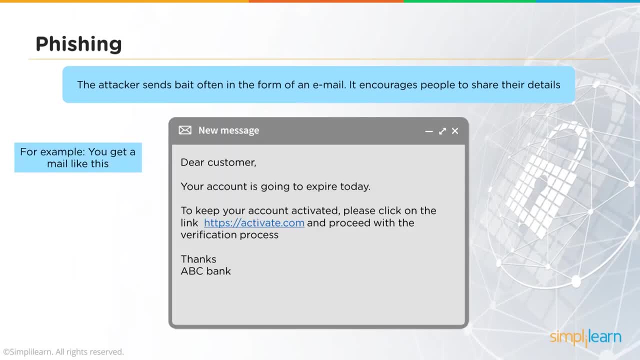 ahead and click on the link and provide that data. So here the example is where the email has been received to your customer. Your account is going to expire today. to keep your account activated, Please click on the link here and proceed with the verification process. 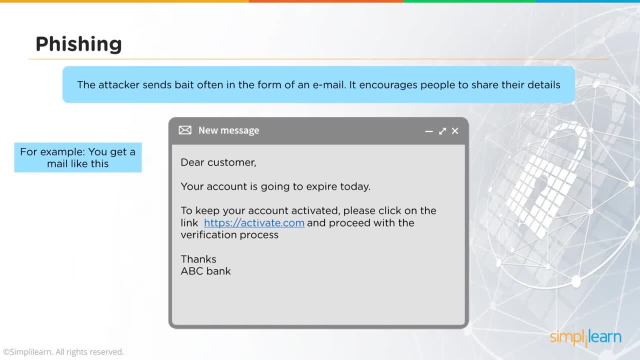 Now, here the link that we see, activatecom would be an hyperlink Which is going to mask the actual URL with the link is going to redirect us right here. The attack is on the gullibility of the customer where they would fear that the account would. 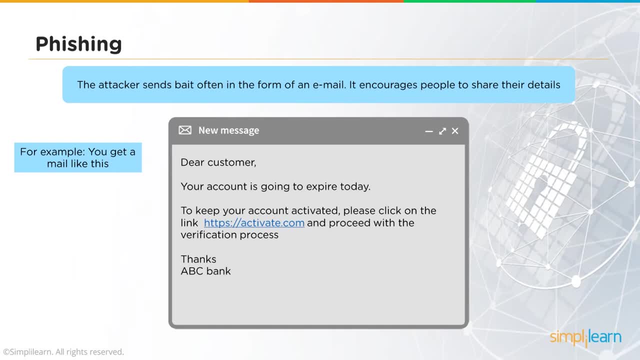 be deactivated and to prevent that, they would press this email, click on the link and then provide the information, thinking that they're just reactivating the account, but they're actually leaking their own information to the attacker. So the first thing you have to understand is banks, or any organization, are not going. 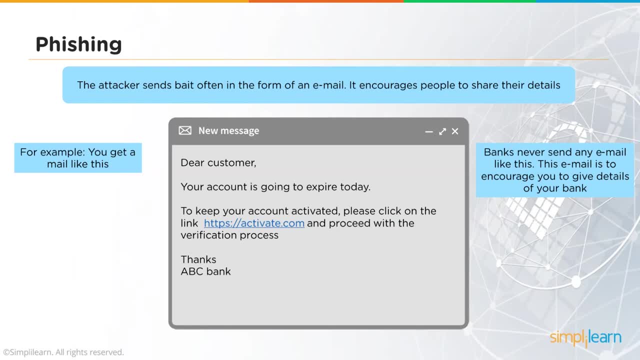 to send you any emails with the link in it Asking you to To reactivate or anything like that. In fact, banks proactively tell us that they're not going to call us and ask for any information. In fact, they would want us to call them on their registered number or the helpline number. 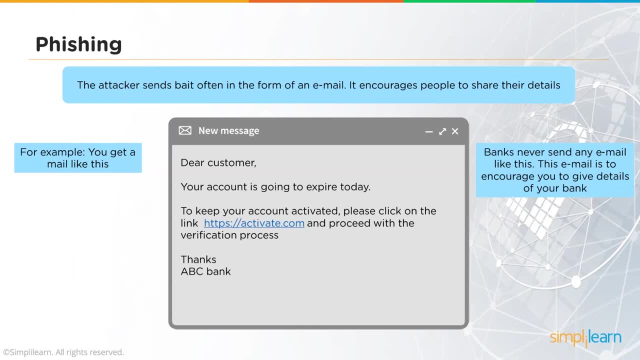 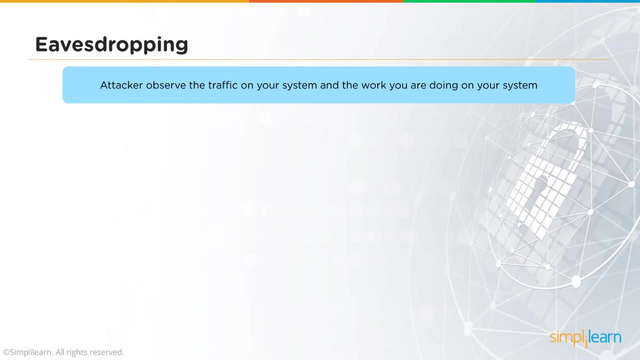 that they have declared on their website or on the cards that we possess. The next attack we're going to talk about is eavesdropping. Eavesdropping is where you observe the traffic on your system and the work that you're doing on your system. 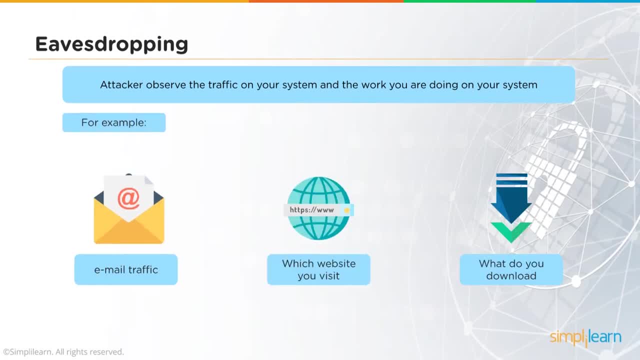 For example, email traffic or the website that you're visiting or what you're downloading. So eavesdropping would essentially be the sniffing attacks on networks, where you're going to sniff data packets and you're going to try to observe the ongoings or the data. 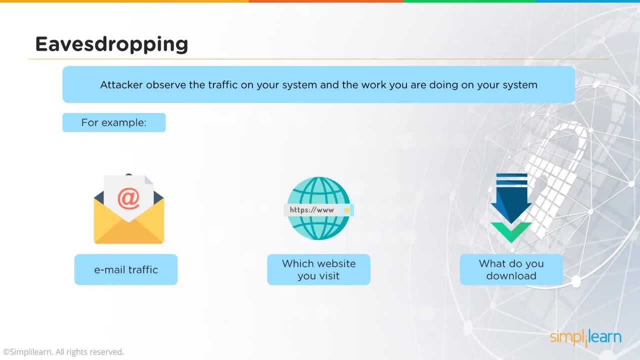 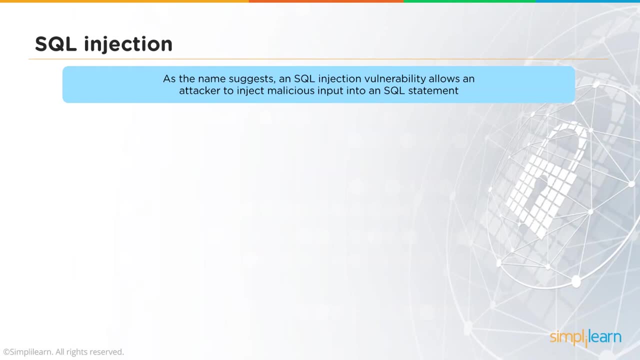 that is flowing between endpoints, between servers, and you're just going to try to observe it. The next attack is SQL injection, or SQL injection. SQL stands for structured query language, which is the language that is used by an application to interact with the database and the database to give that information back to the application. 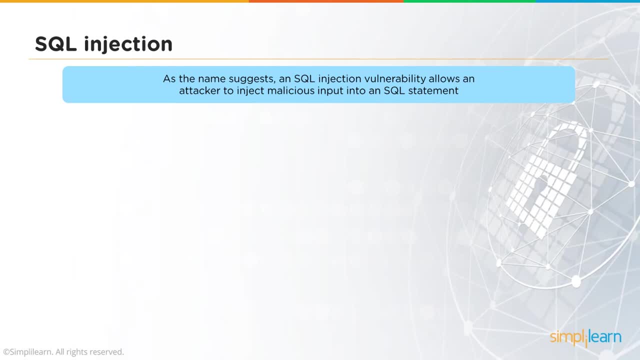 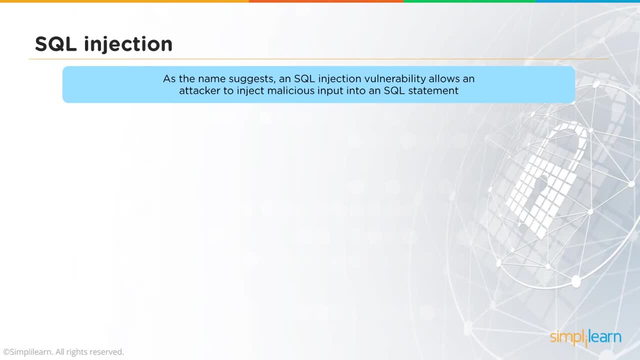 to leak confidential data. especially, they're going to leak data that these users were not authorized to access in the first place. So the next attack would be a password attack, As the name suggests, this attack is used to crack or get the password for users account. 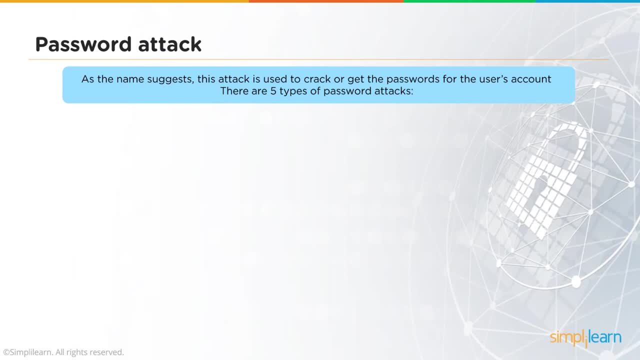 Or when we say crack passwords. this is basically where somebody is trying to brute force, or they're trying to guess the password and they're going to break the password, thus getting access to your accounts. There are five different ways passwords can be cracked. 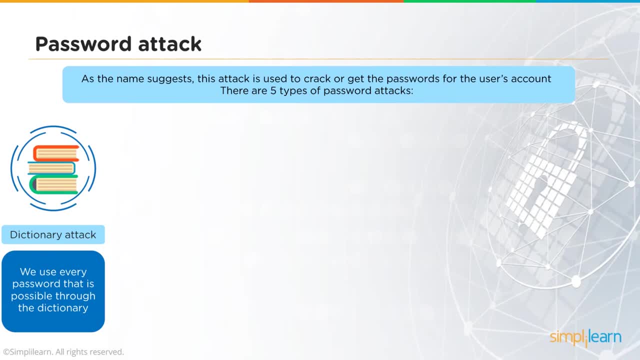 The first one is a dictionary attack, where we use every password that is possible through the dictionary. Now, this is the use of an actual dictionary and that's one of the reasons when we try to create passwords. we are advised not to create passwords based on dictionary words. 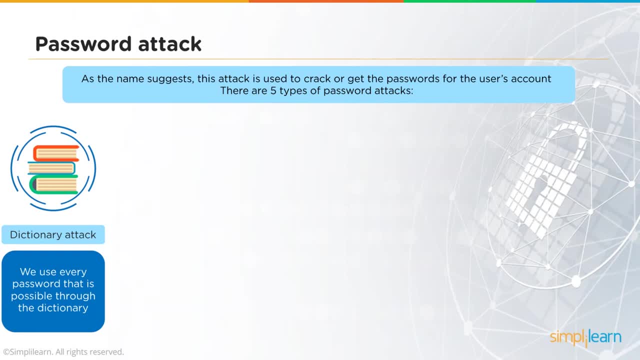 because these are easily guessable and there are lists already out there that contain all of these words. There's a tool that you can utilize, And that tool will then pass through each and every word that is in the dictionary file and then compare it to a possible password. 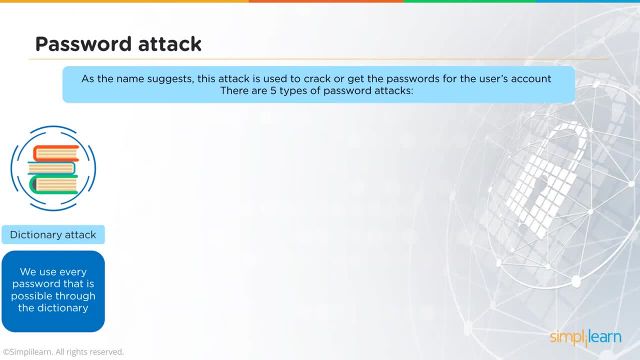 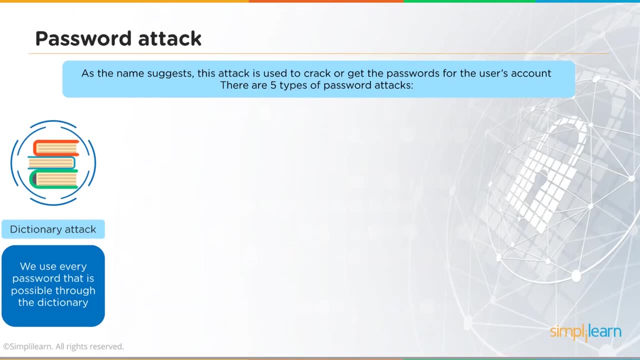 If one of the words matches the password has then be compromised. So if you're observing a little bit higher security, where we have created a password that is not based on a dictionary word, then we want to look at other attacks like brute force. 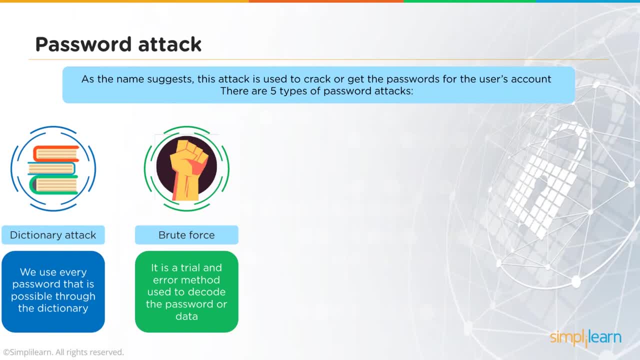 It is a trial and error method. So basically, what we do is we identify how the passwords were created. For example, in today's world, the policy would be to consume in a password any of the alphabet characters A through Z, uppercase or lowercase, 0 through 9, and then special characters. 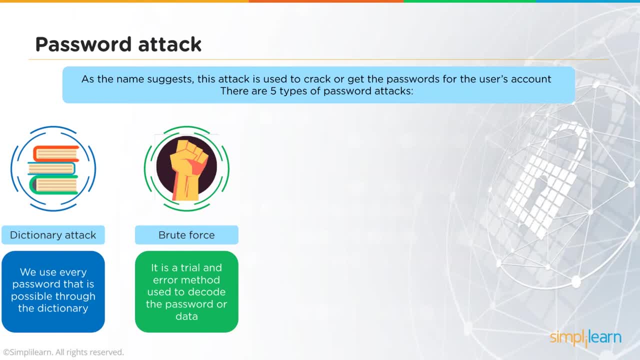 And then we want to randomize the usage of these characters so that they are not easily guessable, But a brute force attack at the same time would then try every permutation and combination that is possible in the entire character set and then try to figure out the password. 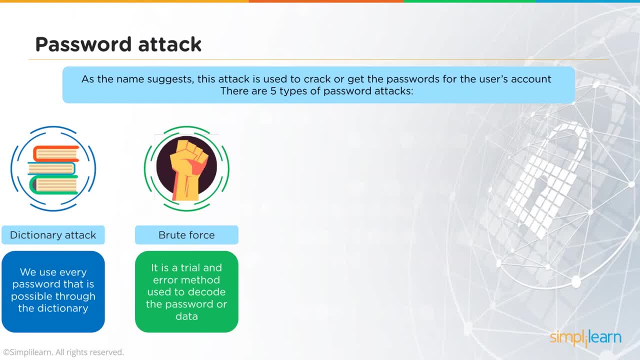 Now this takes a really long time and does take a lot of compute and storage power, and the botnet example comes in, comes back in the one that we saw earlier, which was used for DOS attack. But similarly, if I've infected multiple computers like this, I can then distribute this attack. 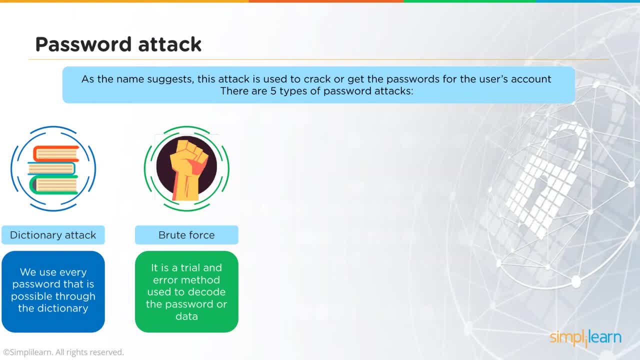 onto all those computers and use the entire compute power that is available to shorten the time that is required to crack the password Now based. this is 100% successful given the time that it may take. So if the time that is going to take is going to be a hundred years, the attack becomes. 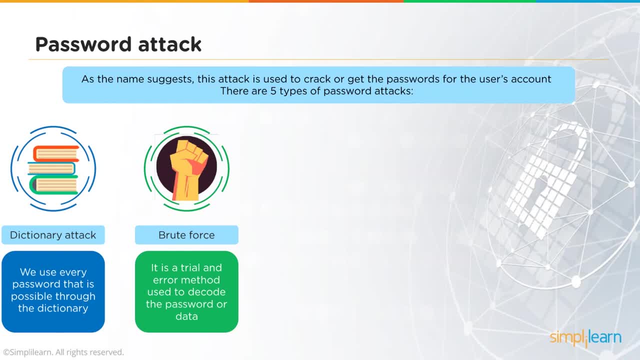 unsuccessful Because during that period the password is most likely to be changed, the technology is going to be changed, and so on and so forth. So if the password is easily guessable, this can be a very easy attack to perform. Then a key logger, which is a similar attack to what we have seen. 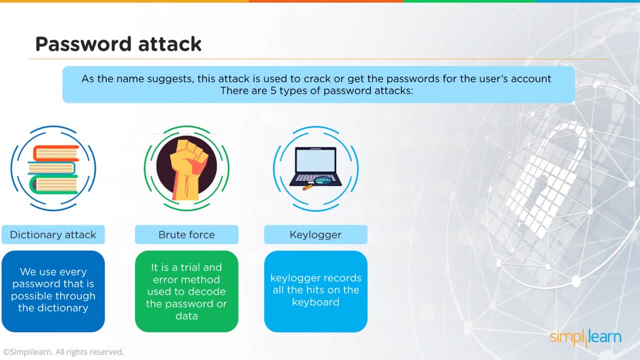 So a key logger, as discussed earlier, is nothing but a software that, once installed on your machine, would grab each and every keystroke that the user has made and store it in a file which the hacker can later on access. So, whatever you have been typing- passwords, credit card information or anything else- 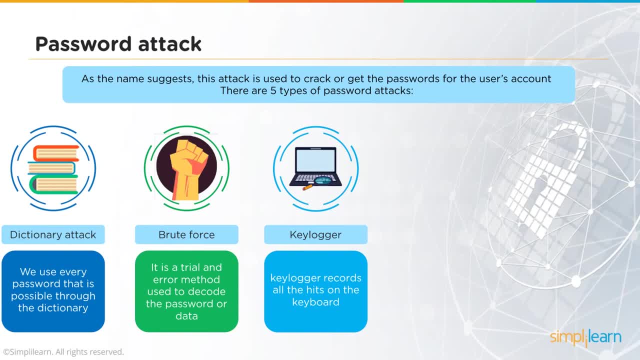 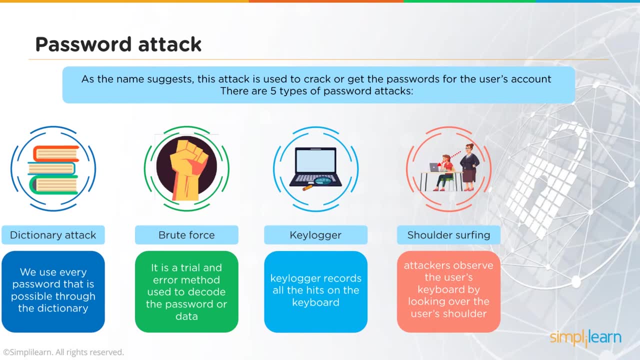 all of those would be recorded and stored in a file, And that's one of the best way a password can be compromised. Then shoulder surfing. This is a physical attack rather than being a technical one. Here you need to be physically, be present when the user is typing in their password. 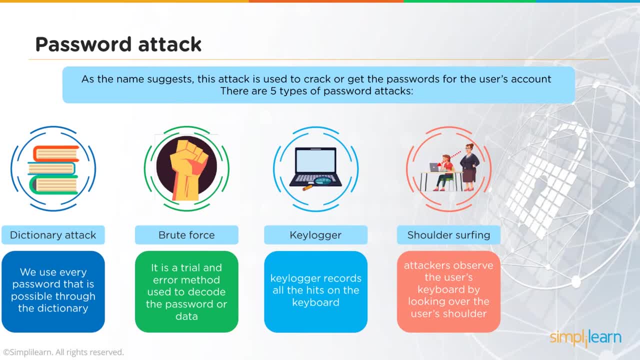 and you actually look over their shoulder to see what they're typing and try to figure out what the password is. If they're quick typers, it is going to be a little bit more difficult. If they're slow typers, it's going to be that much more easy. 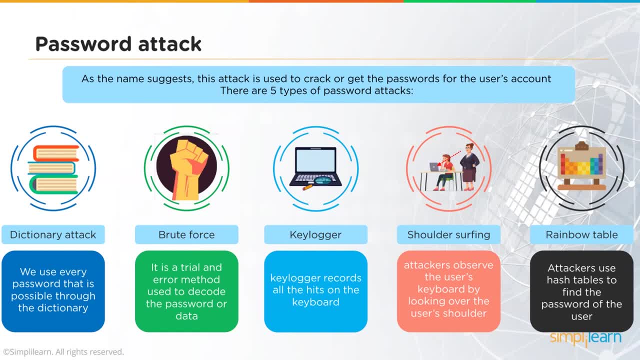 And the last one is called a rainbow table. Now passwords, when applications store them, are stored in hash format. Hash is nothing but a one way signature that is created of the password file, of the word that is used for the password, And it is based on an algorithm. 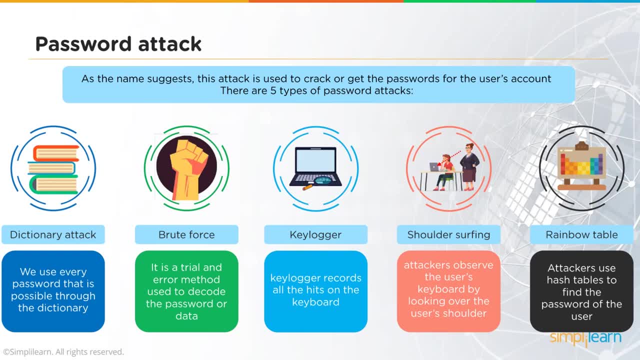 So the input could be a variable length. for example, a password would be seven to 14 characters, But the output of a hash value would be fixed based on the algorithm that you're consuming. So most common algorithms in today's world that we utilize are SHA, secure hashing algorithms. 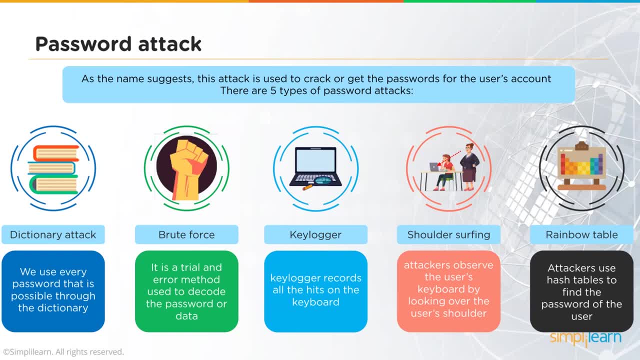 Before that we use MDF. So all of these convert the passwords from plain text into a hash value and store it into a database. So if you actually attack that database to grab a password, you're going to get the hash value, not the password in clear text. 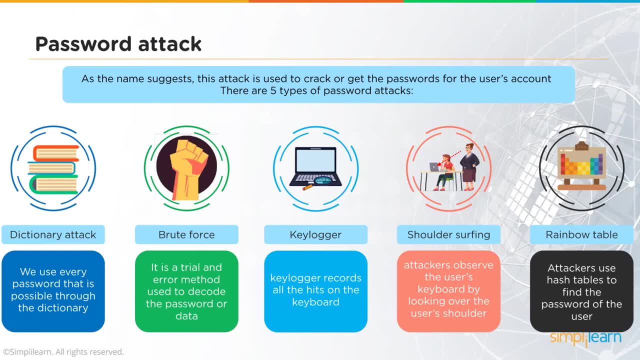 And thus, in that scenario, comes the rainbow table to the rescue. A rainbow table is nothing but a file that will have a list of all possible passwords, along with their hash values in the required format. So, if you remember the dictionary attack, the dictionary attack was nothing but a list. 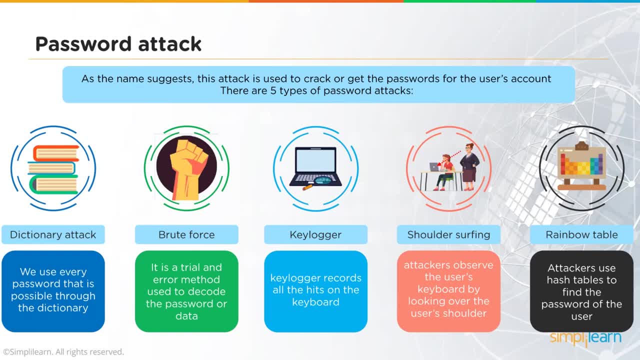 of words based on the dictionary that was stored in a file And then the software was just trying each and every word against a possible password. Here we do not have the word, but we have the hash value. So to reverse engineer hash value, what we created is we created a rainbow table, whether 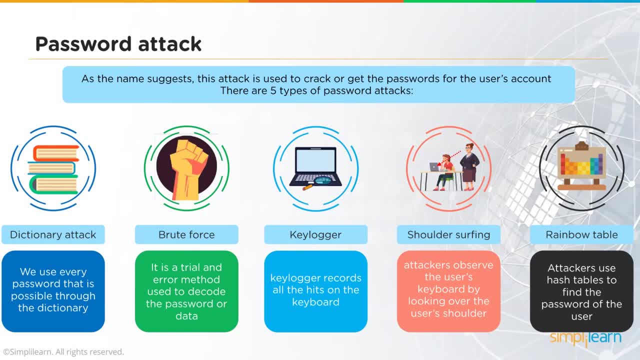 we will list off for the possible passwords and their corresponding hash values. So we then compare the hash value that we have captured and then search for that hash value in the file that we have created, The hash value that matches the corresponding word to it. 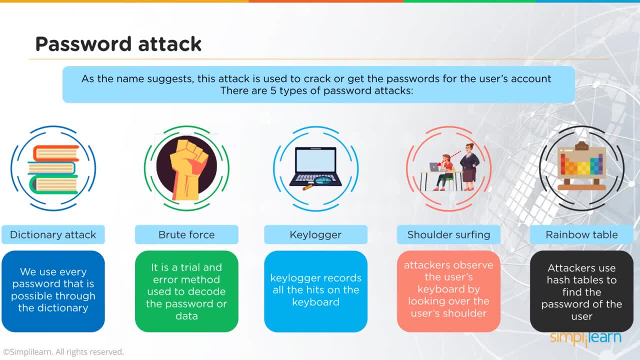 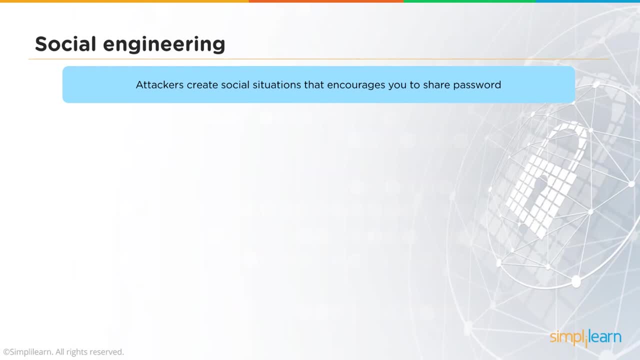 Is the hash value? Is the password in clear text? So these are the five types of password attacks. Then, moving on to social engineering, This is something very common in today's world. This is basically where the prey is the human itself, And the reason social engineering attacks are very successful is because of the gullibility. 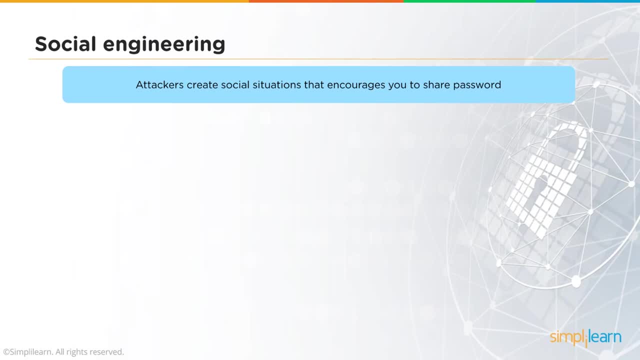 factor that a human has. For example, human has something called emotions that a machine wouldn't. You could plead with a human for a password to be reset by gaining sympathy or empathy, But try doing that with a machine. Those attacks are going to fail. 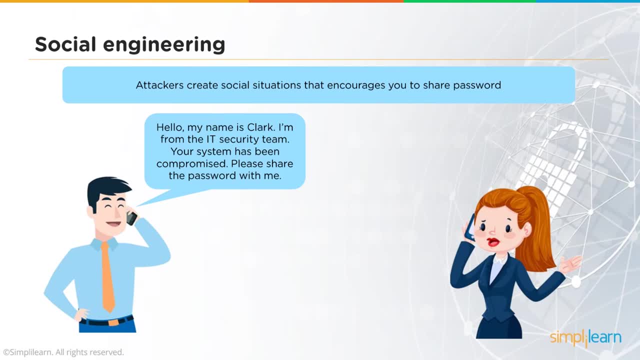 Social engineering attacks are not only limited to those, but we can talk about phishing. Phishing is also a part of social engineering attack, where the gullibility of the user to click on that link is being exploited. In this scenario here, this is Clark. 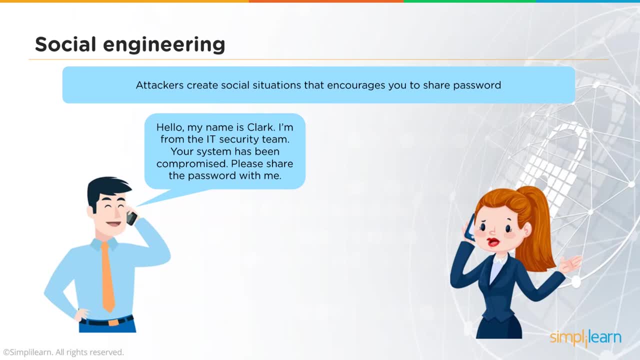 He's calling from the ID security team. That means that he is impersonating, probably, and then telling the victim that the system has been compromised. Please share the password with me. The victim, on the other hand, thinks that the person is trying to help her, probably. 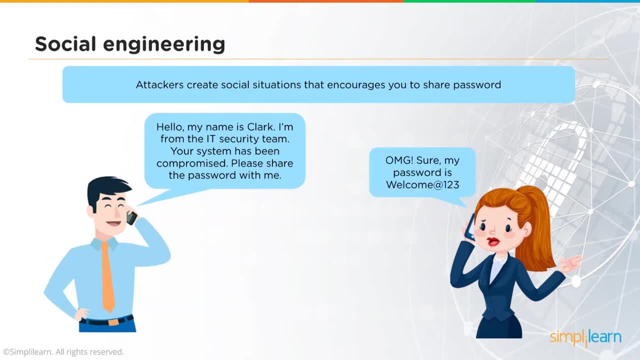 doesn't verify. So he calls the person, press that person and then provides the password over the phone. Now here it is fear that is being exploited, because the password being compromised would clearly upset the end user for loss of data or for the computer revealing confidential. 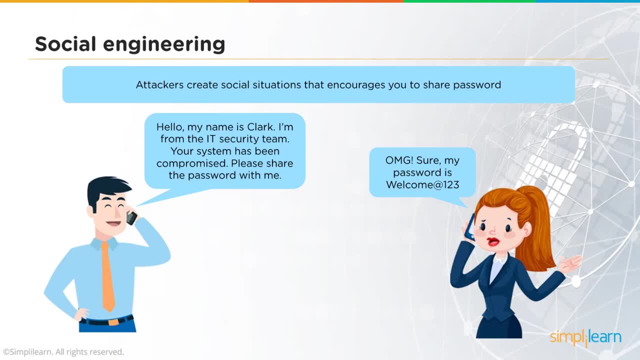 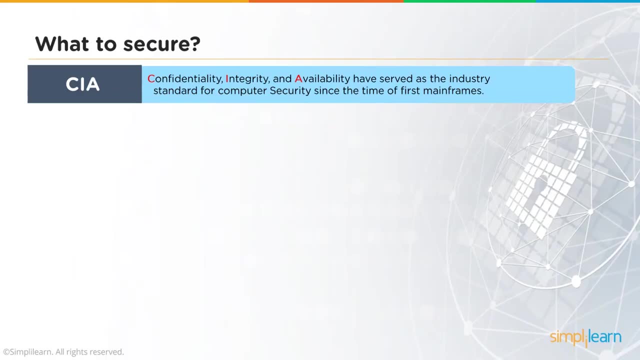 information. Thus, here she is, trusting the security team for the password to be reset and given back to her. Now let's talk about what to secure. when we talk about security, we talk about the CIA, triad, CIA, But CIA stands for confidentiality, integrity and availability. 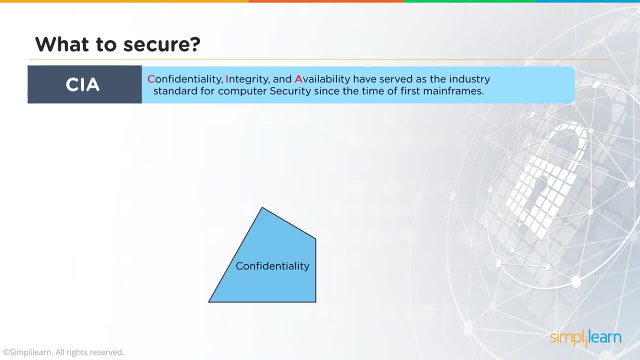 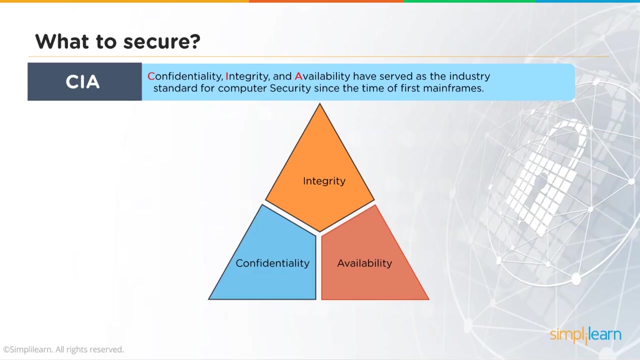 And this is the basis of which your security stands. So any course, any training that you go through will always talk about confidentiality, integrity and availability, And this is the triangle, or the triad, that we're talking about. So when we talk about CIA and we talk about confidentiality, confidentiality is the aspect. 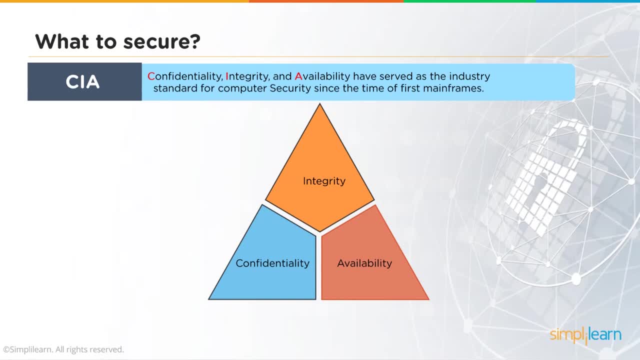 where we want to keep the data secret, based on the value of the data to us. For example, there would be data that is publicly being displayed, For example, the data that we publish on our website which, when a user goes on, is clearly visible over there- but there would be some data that the company needs to keep. 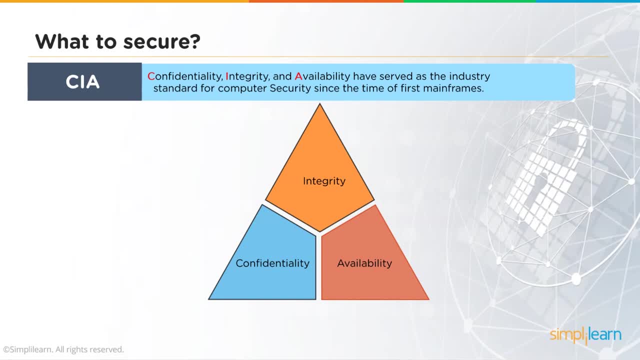 private or within themselves, so that the data would have proprietary value to that organization and that could be sold as a business. Even within an organization, when you're talking about data, there would be classification levels. There would be data that would be made available, depending on the hierarchy and the roles. 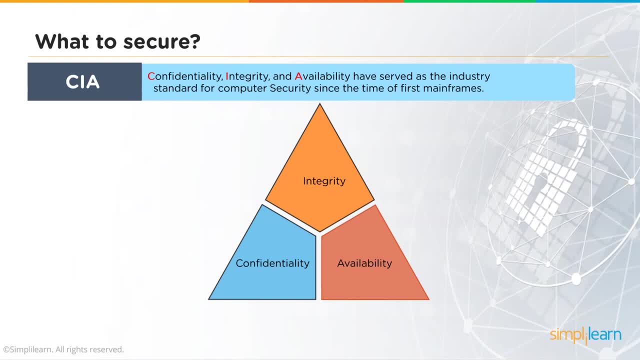 of people within that organization. So when we use those access control lists And we try to keep data available only to those authorized users when they want it, That's what confidentiality is identifying and classifying that data in such a way that the data is available only to authorized users as and when they want it. 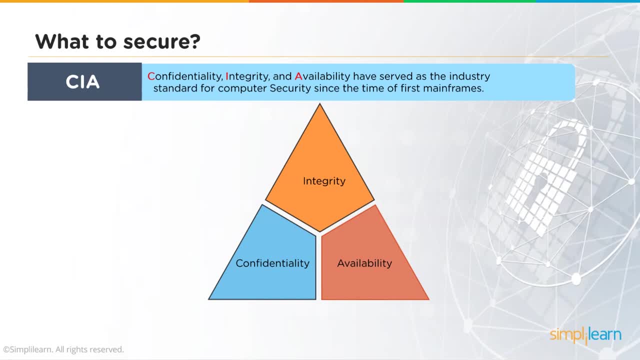 Now integrity is the part where we want to keep the data trustworthy. Even if somebody is able to access it, or allowed to access it, they should not, in an unauthorized or an unintentional manner, be able to change that data without it being audited. 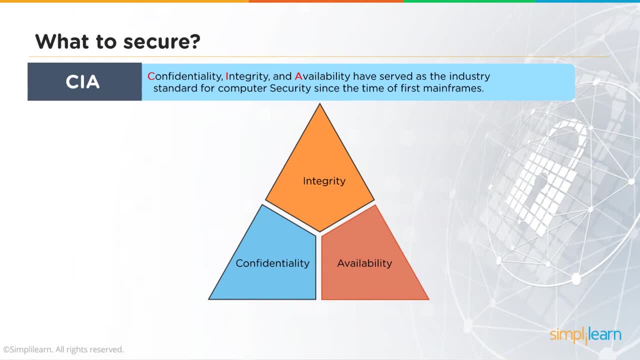 There would be mistakes. There would be mistakes that a person commits at some point in time where those mistakes also need to be weeded out, because mistakes can basically alter the data in such a way where it wouldn't- it would stop making sense. So the integrity part is where we are trusting the data or we are ensuring that the trustworthiness 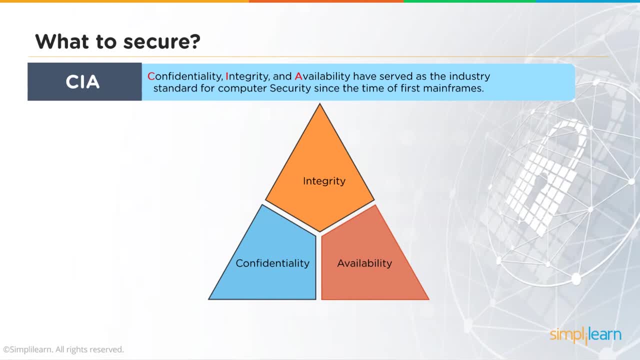 of the data is intact, so that consumers, when they connect to that data, they can rest assured that the data is valuable and is correct at its point in time. The availability part is where keeping the data confidential and its integrity. We still need to ensure that the data is available to all authorized users as and when they need. 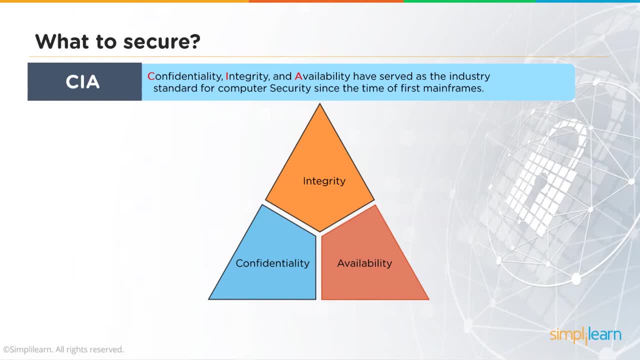 it. So this is the three aspects that you're going to use. Confidentiality: the first defense for confidentiality is using proper access control lists So we decide who's allowed to access the data and who's not allowed to access that data. Once we have created the authorization, we want integrity verification mechanisms for 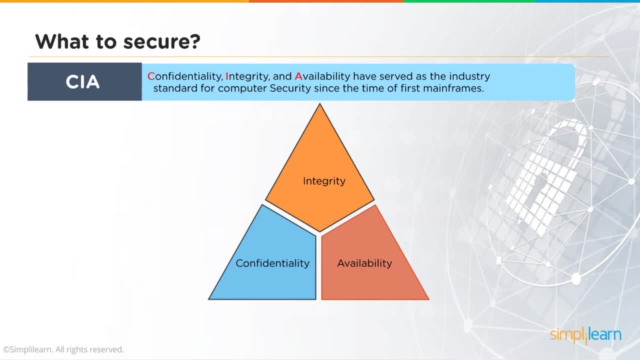 example, hashing. So we have some data stored, we create hash values of that data and we store them in a secret file. So we keep on taking the hash value of those data to see the match. So if the hash value that we have taken now matches the hash value that we had taken earlier, 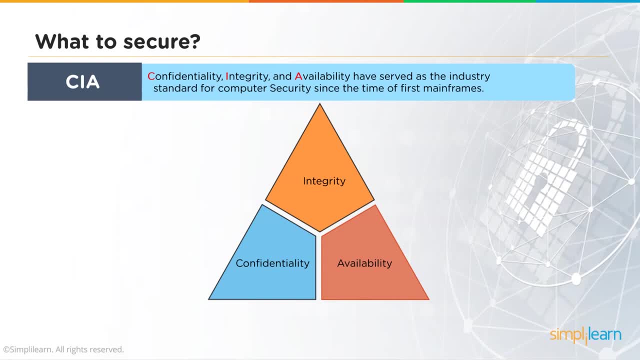 the data is still intact. It has not been modified. But if the data gets modified, even by a single character, the entire hash value changes. So if the hash value of the current data does not match the hash value of the of the data that was taken before, then the integrity is no longer there. 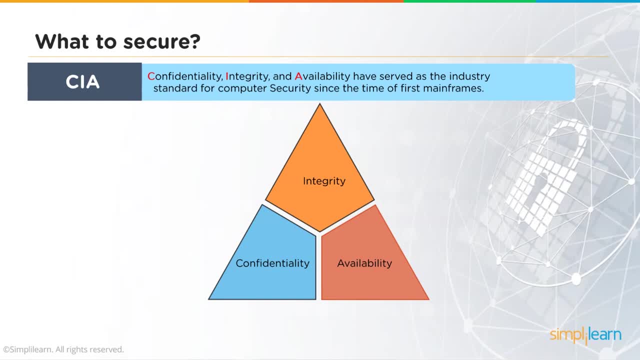 Now, integrity verification cannot be done on files that keep on changing often. Normally we will use system critical files or some very secret files that remain static and do not change often. Only then can we take hash values and then we can compare them properly to. 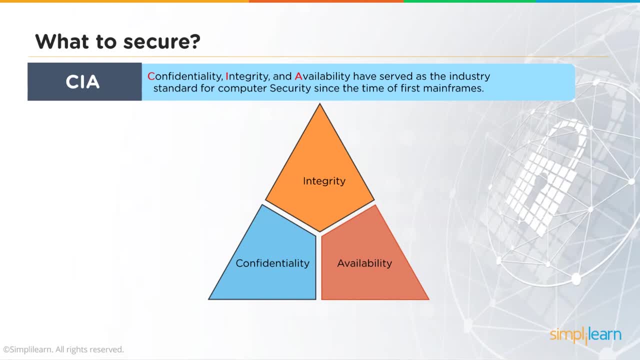 see if they have been modified or not. The availability part is creating redundancy, The infrastructure in such a way that even if there is a small failure, we can absorb the failure, we can still move on and still that data can be made available to the end user. More tips behind. 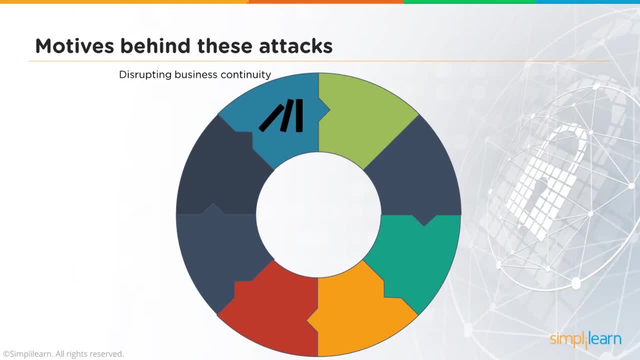 this attack. Let's discuss more tips behind these attacks. The first motive of any attacker, especially when you have discussed denial of service or distributed of denial of service, would be to disrupt business continuity. If there is an interruption in the continuity of a business, it would cause great harm to the organization, Let us say lost profits. 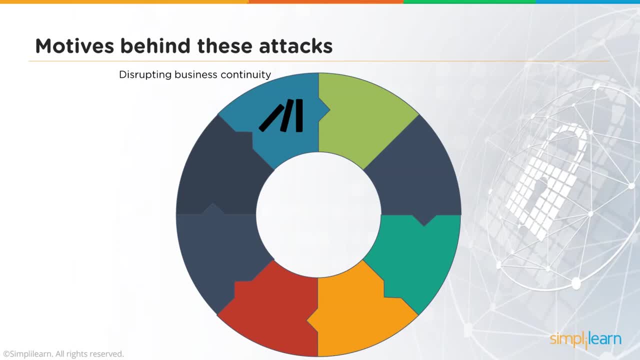 businesses revenues, loss of goodwill, service level agreements not being adhered to, which would cause losses to the organization, And so this is a good sign, because, least ort of those possible, tässä leads to a morale coil which might not be supported at all. refused time for one reason or even be brought into existence. If the sale So, the business350 tab series is considered as such as long as there is a total tops 20% out of the 25% market cap � and 60% left in percent. 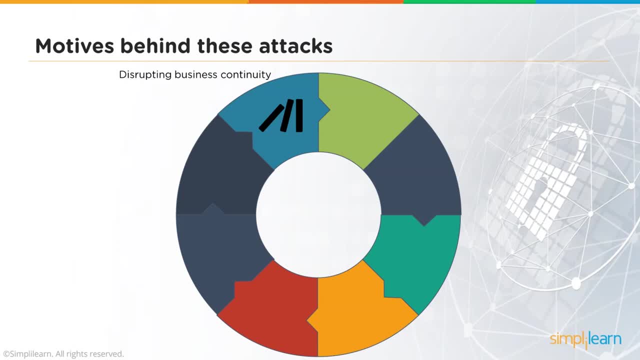 cause penalties to be paid to the customers and the clients, and so on, so forth. Apart from that information theft and manipulating data, hackers normally would steal information from organizations and then would try to resell them on the black market or to competitors so that they can make a. 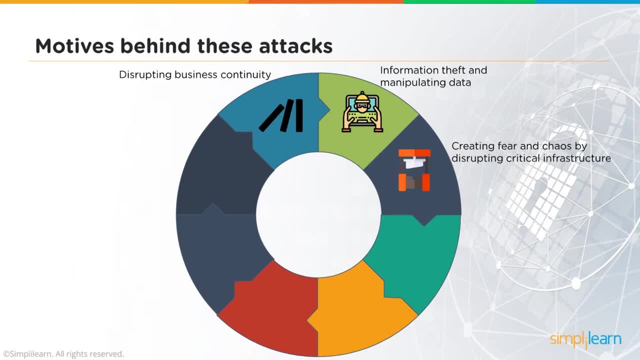 quick buck, Creating fear and chaos by disrupting critical infrastructure. This is where terrorist hackers could attack organizations or could attack governments, crippling some of the services that they provide to the nation or to some particular areas, thus creating fear and panic amongst its citizens and thus harming the nation as a whole. Financial loss to the target We have. 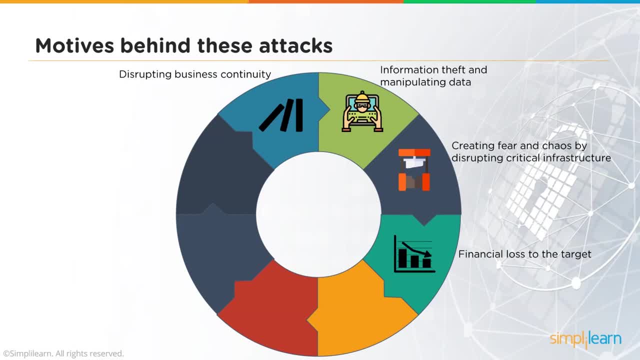 all talked about banks getting hacked, money being stolen from their individuals, getting compromised by phishing attacks and losing their life savings. Similarly, organizations can also lose a lot of money if they get hacked, especially with the new laws in the market where they may have to pay penalties. 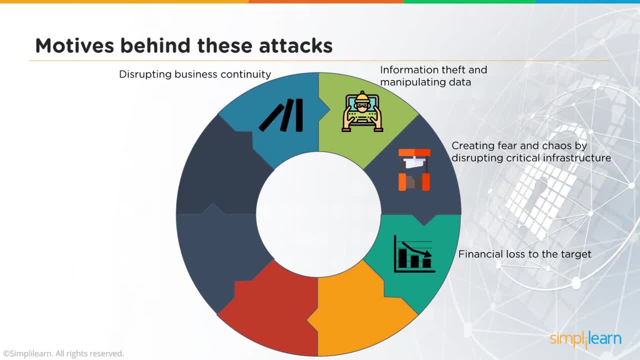 Not only to the customers but to governments, for failing to protect particular data Achieving states military objectives. Countries keep on spying on each other. We have heard a lot of news in the recent world where a specific country like Russia was supposedly involved in the US election. 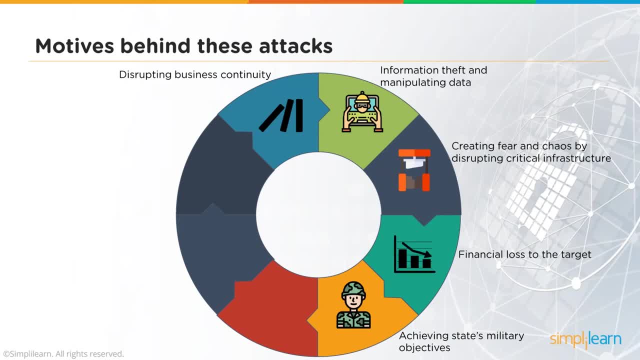 and so on, so forth. So some of these attacks could really happen in the world. In fact, if you take a look at some of the recent news in the US, you will see that the US government is trying to create a nuclear strategy that they had created and what flames and Stuxnet created as a havoc, as 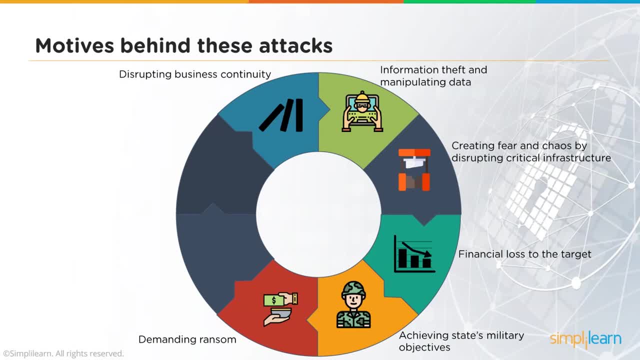 far as Iran's nuclear reactor was concerned, Demanding ransom. This is a very recent case in 2017, where WannaCry was released to the world and it infected a lot of computers, costing the world around four billion dollars in losses, Damaging reputation of the target, Loss of goodwill. You wouldn't want to take a look at the? 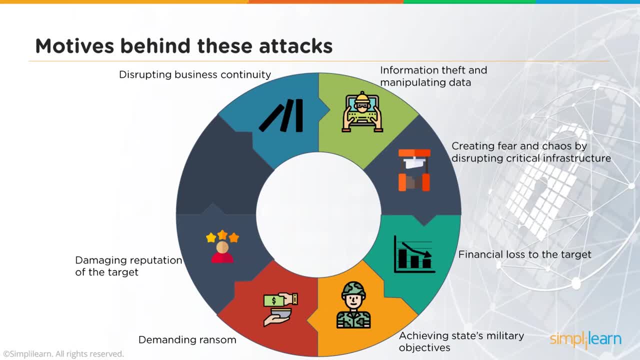 data. You wouldn't want to trust a business who gets hacked right. So I mean the thought processes. if you cannot secure yourself, how would we expect you to secure critical data or sensitive data of your customers? And then propagating religious or political beliefs? We have? 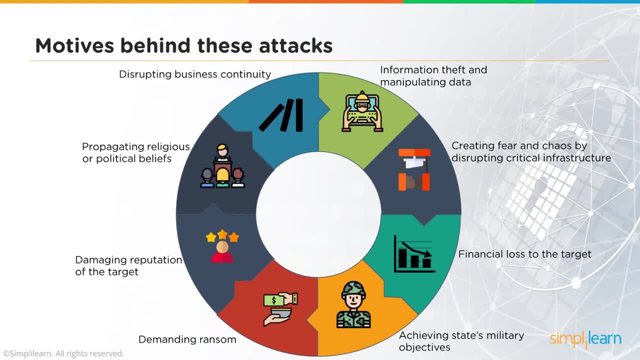 organizations like ISIS, who have a lot of propaganda online, a lot of videos, audios, where they keep on targeting people who are susceptible to these kind of videos and try to recruit them for their own, for their own causes. So these are some of the things that are happening in the world right now. 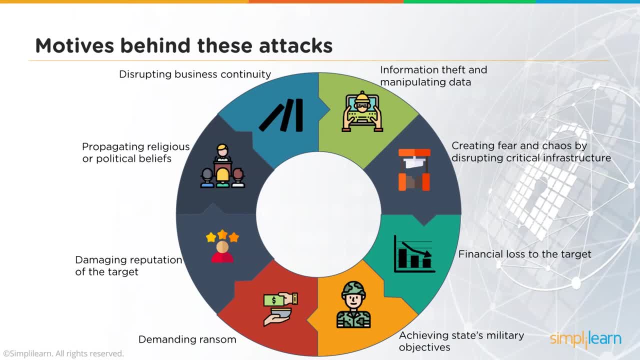 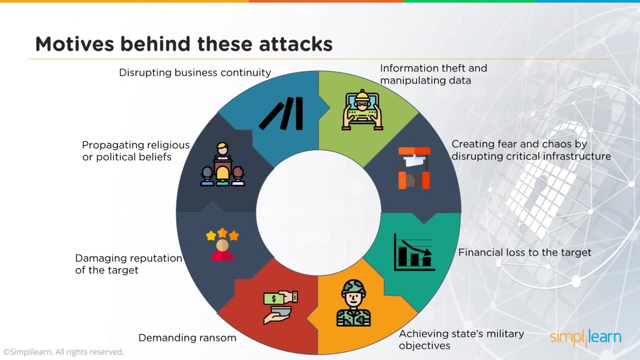 Some of the motives behind these attacks. A motive could be anything. For example, an hacker could just be doing it for fun. Maybe somebody is just trying to hone their skills or learn new skills and they just try to try it out against a particular victim, without the victim. 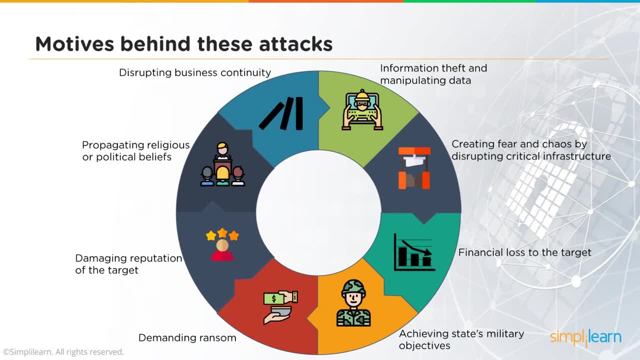 even being realizing it, or the hacker actually having nothing against that victim. So a motive could be anything and everything that you can think of, of anything that would encourage a hacker to attack a particular organization. So I think it's a very important thing to think about. 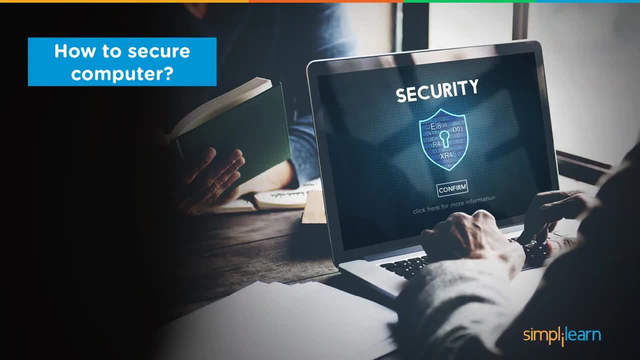 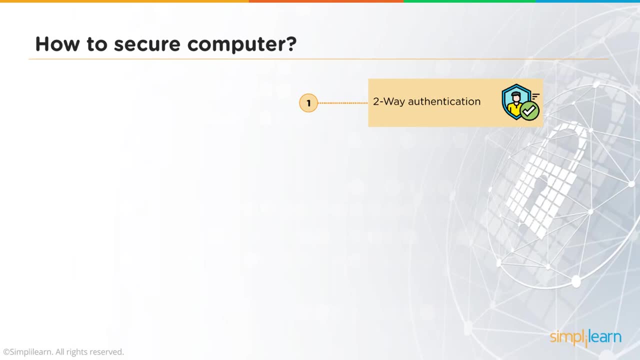 Now let's talk about how to secure a computer. Now there are multiple ways of securing computers. These are some of the basic ways. We are not going into advanced ways. We are still not talking about data centers. We are looking at end users. We are looking at talking and talking about securing. 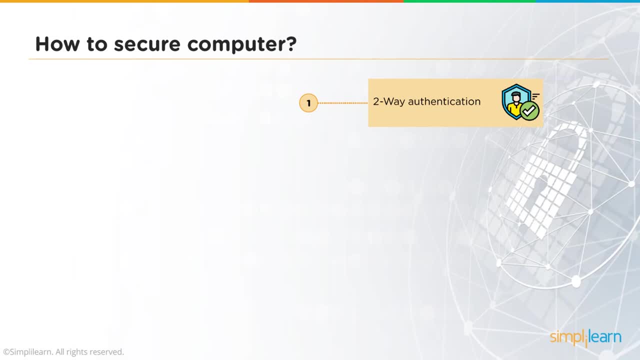 computers. So the first and foremost is a two-way authentication mechanism. Most of us use that on a regular basis. We have secured our Gmail and Facebook accounts with two-way authentication, where we use usernames and passwords. We have secured our Gmail and Facebook accounts with two-way authentication, where we use usernames and passwords. 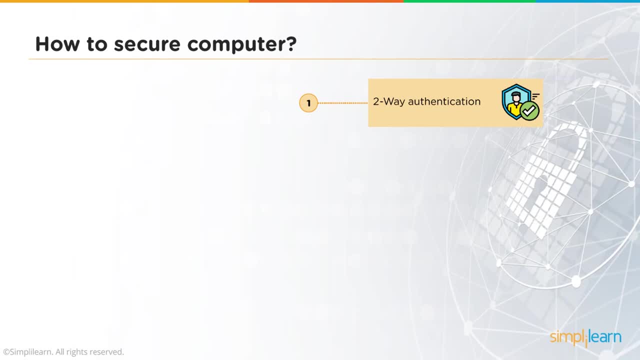 And then an OTP, or a one-time password is texted to us or sent to a particular email address, which we then have to input to then get access to the required resources Securing passwords. we also have been told quite a lot number of times that passwords need to be secure, which means that they 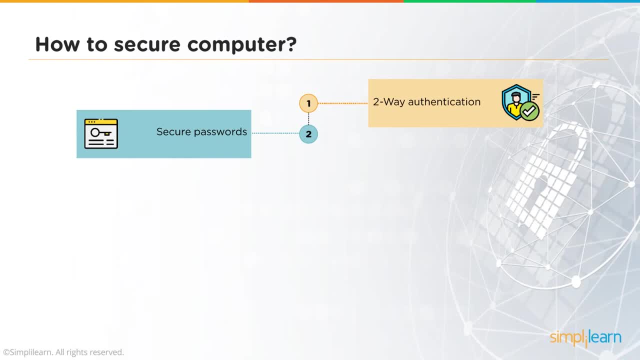 should not be easy to guess. They should not be based on names. They should not be something dear to us, Shouldn't be a reverse of a mobile number or a combination of date of birth and the mobile number. Basically, a password should be randomized, should be of a length of not less than 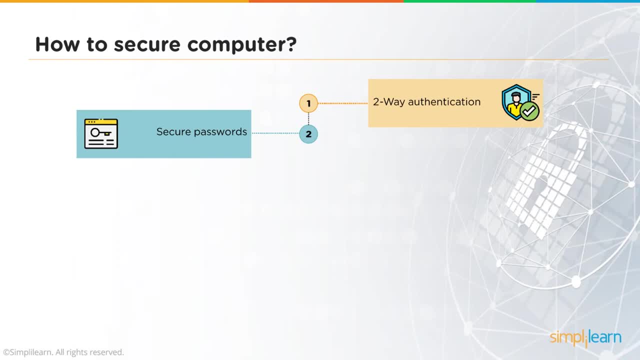 eight characters. 26 characters is supported, so it depends how much you want to secure your password with. Again, there are so many passwords to remember. that's where we actually start lacking in our password creation skills, where we use a same password for multiple accounts or then create. 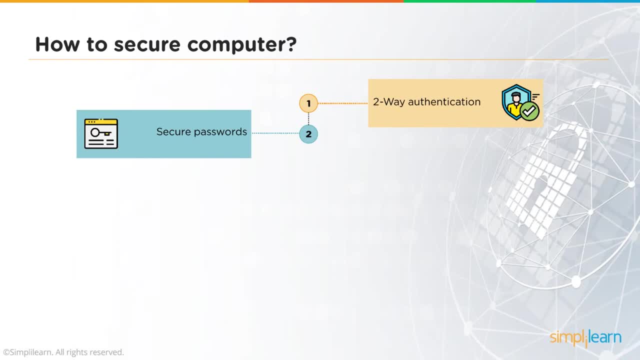 a password that we can remember easily and then use those passwords. But in a sense a password should be randomized, should not be created on anybody's name. anybody's likeliness should not be dictionary based but should be combination of uppercase and lowercase, a through, z, zero through. 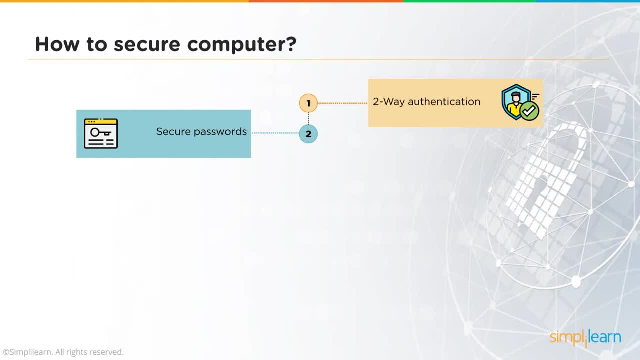 nine special characters and it should be randomized. The string not should not be less than eight characters. can go up to 26 characters maximum. Regular updates. this is very important when we use softwares and we are especially relying on third-party softwares, for example. 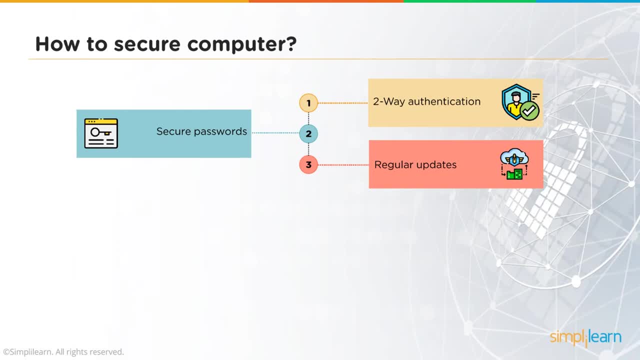 operating systems. For example, if we are using Linux, Microsoft or Mac, there will be flaws and vulnerabilities that would be identified in any of the operating systems on a regular basis, and that is why, when we purchase a license, we get free updates for life of that operating system. as individuals, 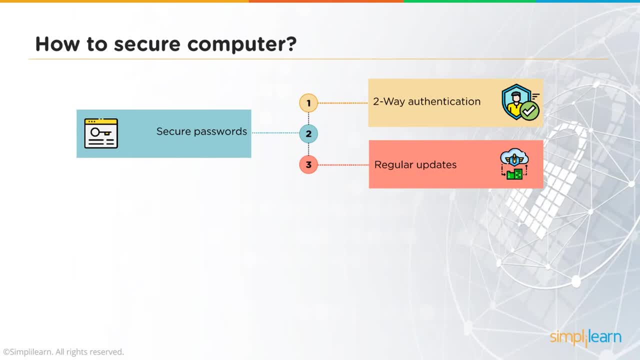 It is important that we keep on installing these updates. these updates may not only be functional in nature, but could also be security updates. for example, Microsoft releases security updates every second Tuesday of every month. updates are collected together. these, basically, are patches that have been created to patch the. 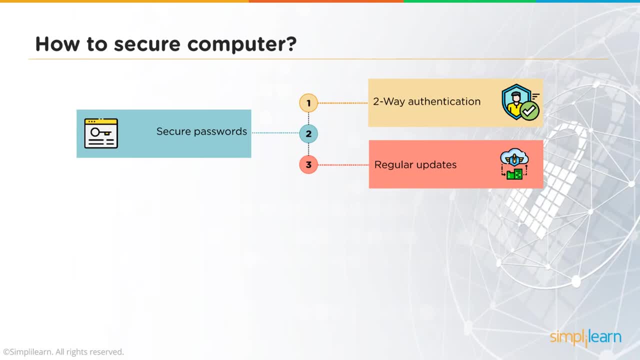 most critical vulnerabilities, the most common vulnerabilities that have been identified not only by Microsoft, but have been reported to them by third-party organizations and individuals as well- and here I'm just saying Microsoft. it could be anything. you could be using a third-party application which you have downloaded and installed. you need to keep on updating it. it could be as: 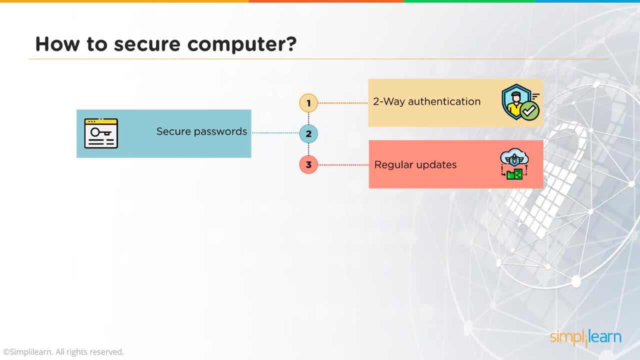 simple as management softwares or maintenance softwares that you have installed on your machines- Microsoft Office, if you will. any software, once installed, needs to be maintained, its patches to be identified and installed on regular basis, so that the most common known vulnerabilities on those applications would be plugged in, thus reducing your risk of getting hacked by an. 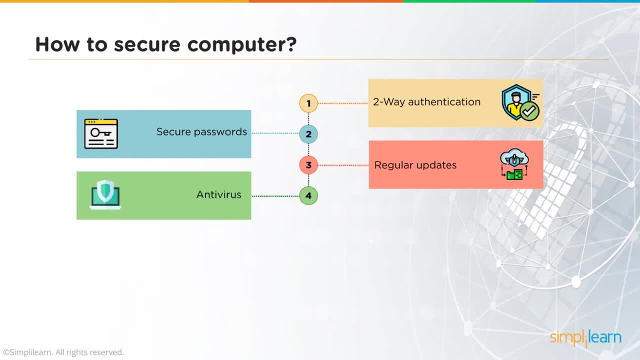 existing vulnerability Antiviruses. in today's world, when we spend so much time on the internet- and we spend a lot of time on the internet- we download all the files with our email, with attachments, and we download a lot of data of the internet. now an antivirus is there to help us to. 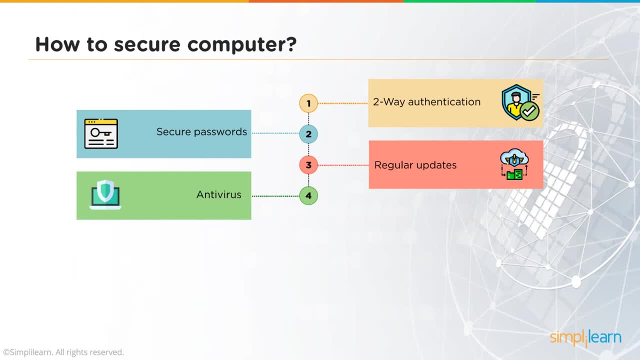 identify whether any of these files that we are uploading, downloading, receiving my attachments, could be malicious or could have a trojan or a virus in it. so the antivirus job is to scan these files and warn us. if there is anything malicious about that file, then firewalls. now what is the? 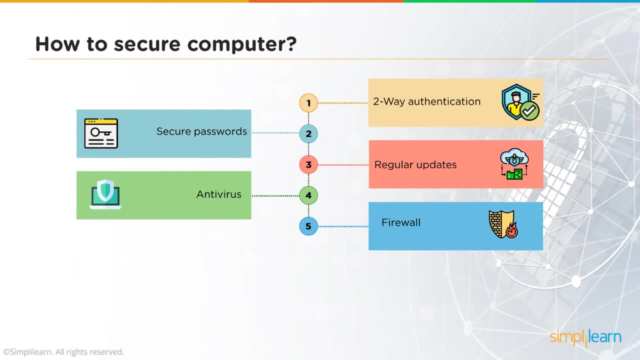 difference between an antivirus and a firewall. An antivirus scans for files and malicious screens and it scans for files, and an antivirus scans for files and malicious screens, scripts or data within those files. Firewall is a software or a hardware that will allow or disallow certain protocols or certain connections from happening, So a firewall is configured in. 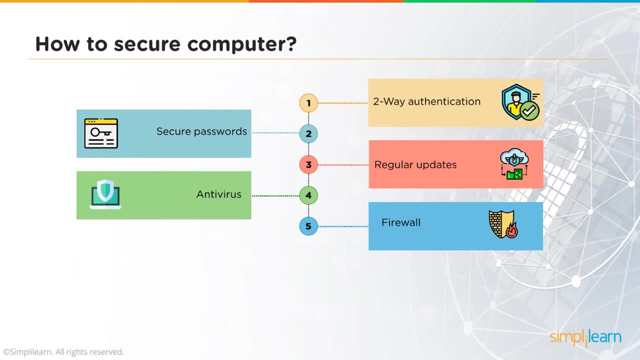 such a way where you allow certain protocols to work, certain ports to be open, certain services to be functional. If a firewall is configured to block a particular service, any incoming or outgoing connection- as the rule may be- will be blocked by the firewall, thus safeguarding the 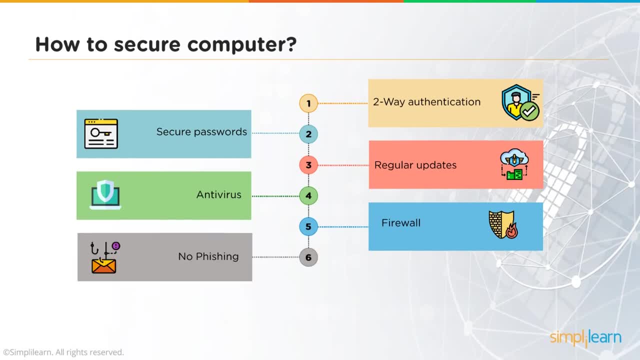 end user from that kind of a connection. Phishing- Phishing attacks- are very common nowadays. There are a lot of anti-phishing toolbars available on the internet. I personally use NetGraph. These anti-phishing toolbars basically look at the sites that we visit on a regular basis and then give us 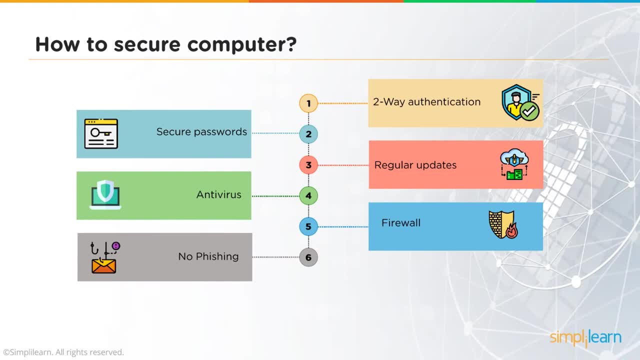 a risk rating of whether the site is genuine or is a probable fake site. On a regular basis, we also receive emails from unknown sources about lotteries that we have won or a Nigerian prince who has lost a lot of money. So these are the kinds of sites that we visit on a regular basis. 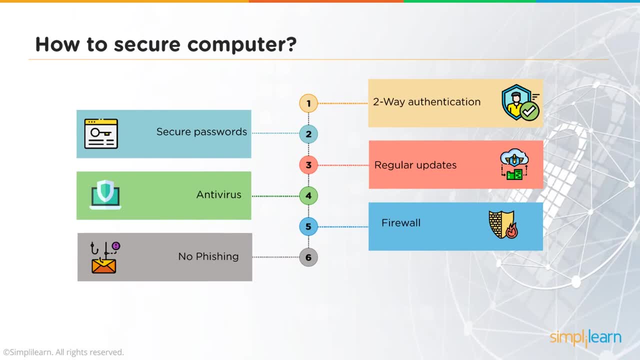 We receive SMS on our mobile phones as well, So we need to first verify the authenticity of these emails to understand whether these are genuine emails or fake emails. How to do that, we'll be looking at that in a future video of how to identify phishing mail and how to identify whether. 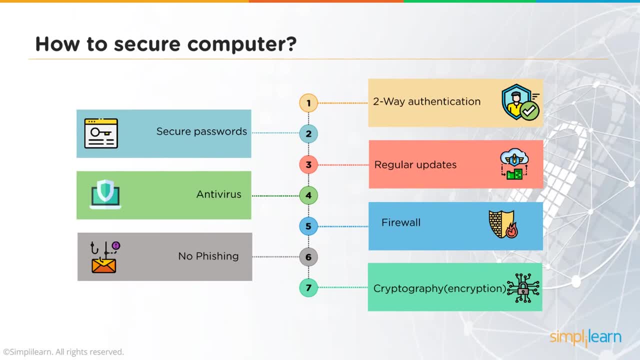 the mail is genuine or not. Try to encrypt as much data as possible, but be aware that with encryption you would be consuming a little bit more compute power, maybe a little bit more network bandwidth and a little bit more storage. So there has to be a fine balance of how much encryption we 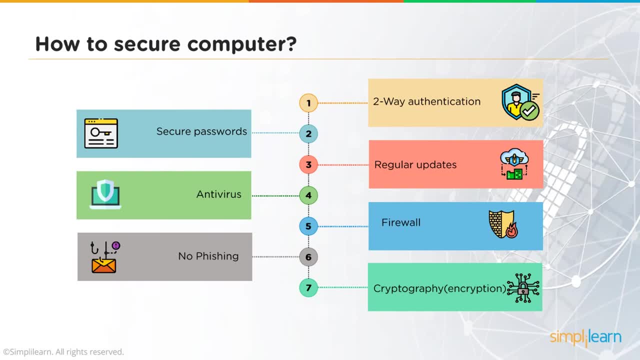 want to use, compared to how much compute and how much capacity that we have. But in today's world, with the latest laptops having at least 8GB RAM and i5 processor being common, encryption is a very good option Once, let's say, an entire volume or a hard disk has been encrypted, even if somebody 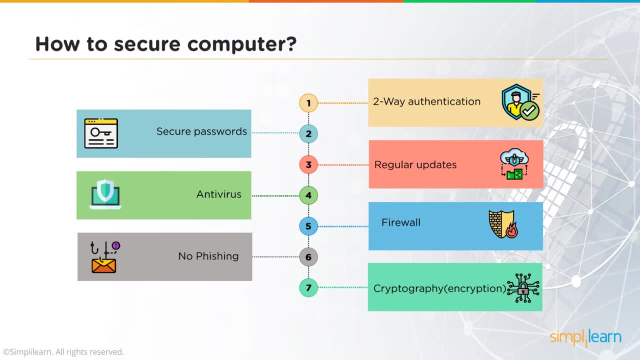 tries to get access to it. they would not be able to understand the data till they crack the encryption key to decrypt that particular data. When we are transmitting data over the line, we always should be using HTTPS. the S stands for SSL or TLS, secure socket layer or transport layer security, which ensures that data is encrypted while it is. 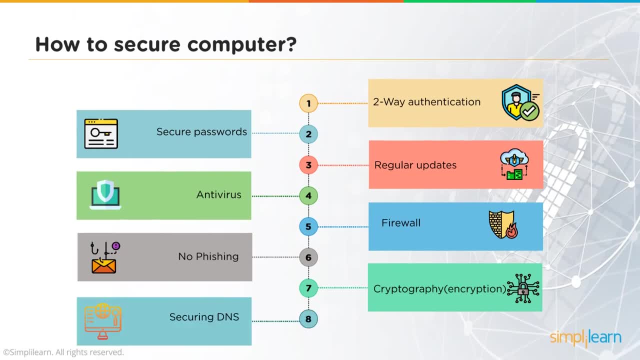 being transmitted over the intranet or the internet, and securing your DNS servers. DNS servers are domain name servers, which are basically indexes that allow a mapping of a domain name to an IP address, For example, when we type in googlecom in the address bar of a browser, the internet. 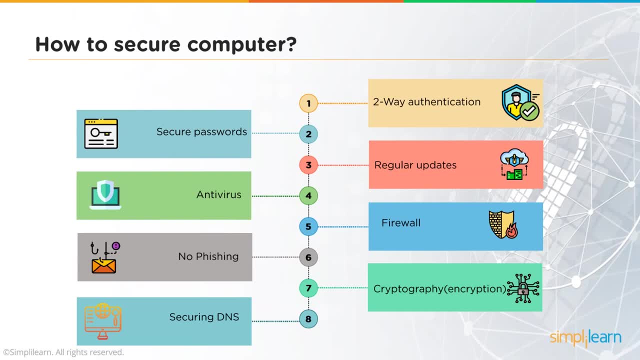 doesn't know what googlecom is. There is a DNS server which would host an index of all the domains with their corresponding IP addresses, and it is these IP addresses that help us identify devices over the internet. So securing these DNS is very important, For example, if a hacker is able to send 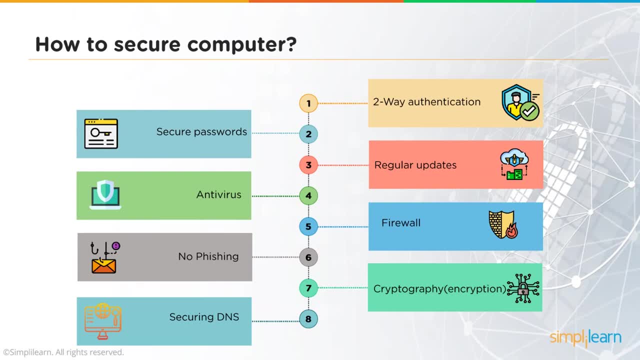 a fake update to a DNS, changing the mapping of a particular domain with a particular IP address, and the hacker then can host a malicious server, give it a particular IP address, change the mapping on the DNS server and thus have unsuspecting users redirected to malicious websites without them even knowing what's going on. So securing DNS in today's world? 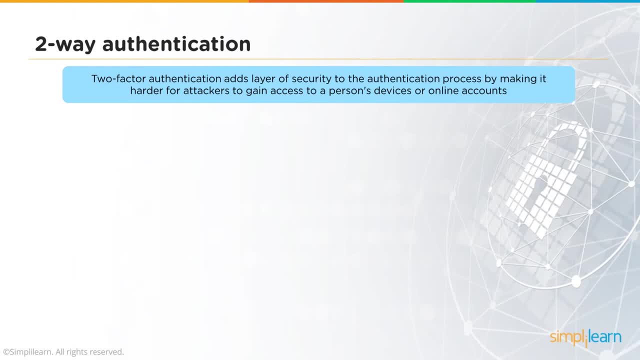 is very much important. Let's go through some slides. Two-factor authentication adds layer of security to the authentication process by making it harder for attackers to gain access to a person's device or online accounts. As discussed, when we use online mechanisms, or let's say, in this example: 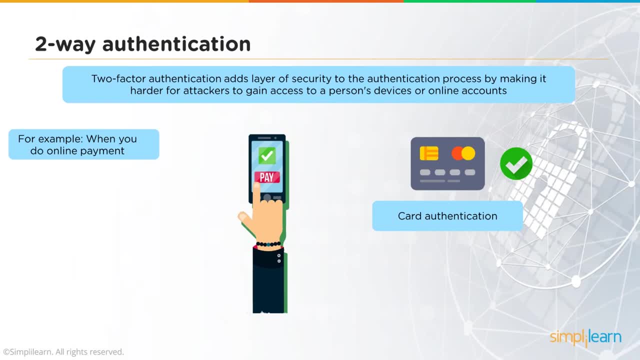 we are using an online payment, and when we are on the bank site, we type in what are the payment recipient is, the amount and all that data, and when we click on pay, we need to authenticate that the payment has been initiated by us, and so the bank sends a OTP or a one-time password to us for. 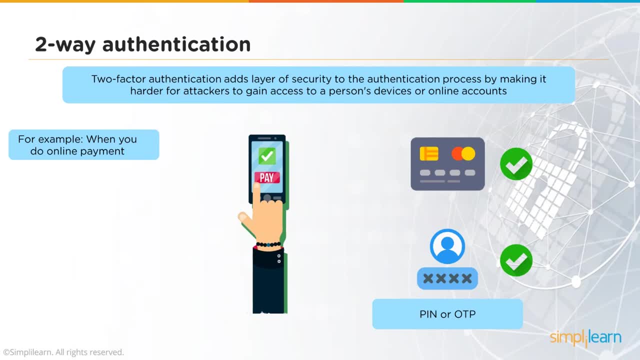 authenticating the transaction right. Once we receive the PIN or the OTP, we type it in the website- on the bank's website, and then the transaction is authenticated. If the PIN or the OTP is incorrect, the transaction gets sent to the bank and then the transaction is authenticated. 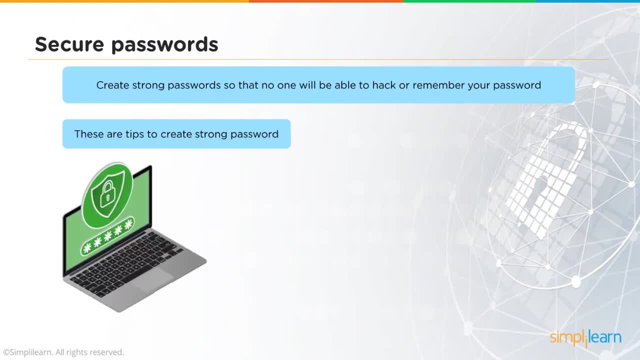 Invalidated right there and then secure passwords. So, as we have been saying, passwords need to be strong, they need to be created in a certain manner which can be randomized. so here we are prescribing at least 15 characters. Now I understand 15 characters of passwords, which 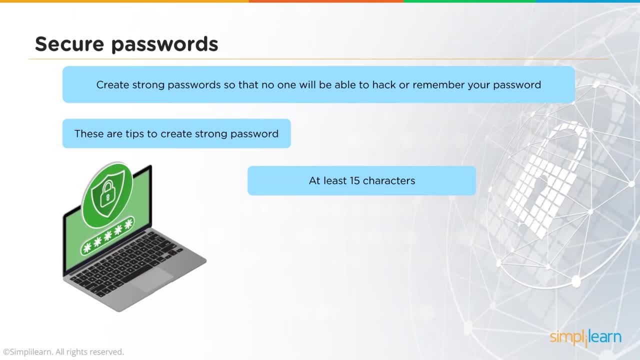 are unique to each and every account. it would be very difficult to remember. however, it is the necessity of the hour, and this doesn't mean that we create very complex passwords and then write them down on a piece of paper and keep that paper in our wallet. that's defeating the purpose. So we 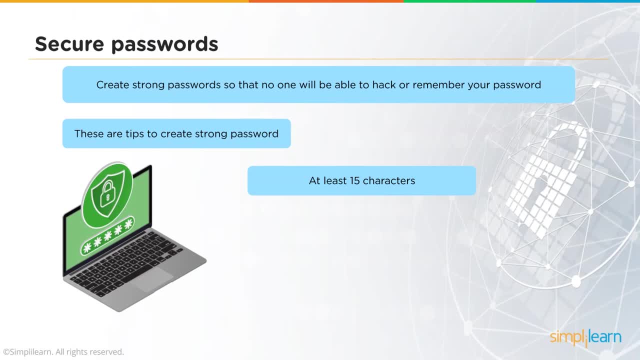 train our minds and train ourselves to create more effective passwords which cannot be guessed or cannot easily be cracked. So at least 15 characters should include capital letters, should include special characters like at the rate, ampersand, hashes or percentile, and should include numbers. So, as we've stated earlier, a password should be a randomized string of uppercase and lowercase. 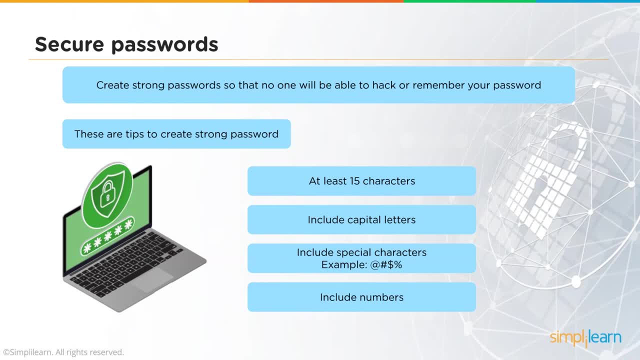 alphabet, a through z, zero through nine numbers and special characters. It should be randomized in such a way that it should not be on a dictionary word, should not be a variant of a particular word. for example, normally we use the word p-a-s-s-w-0 or w-o-r-d as password and then 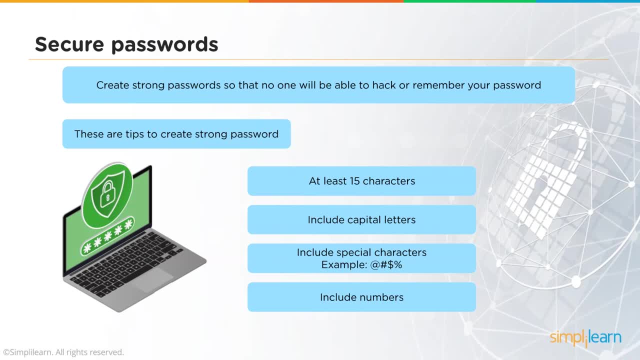 to complicate a little bit, we use the variant p at the rate s-s-w-0-r-d. These are still easily hackable passwords because they are commonly used by a lot of users in the world. so we have to be very careful and we have to create those passwords which are unique to us. 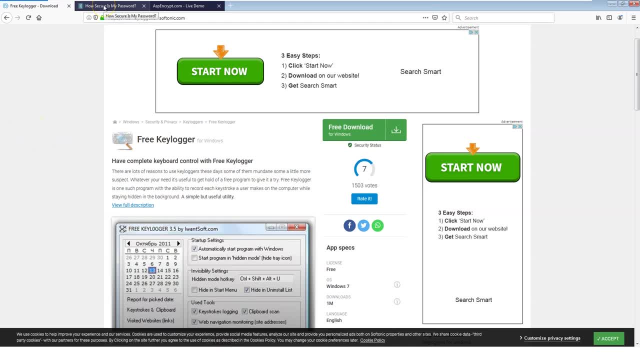 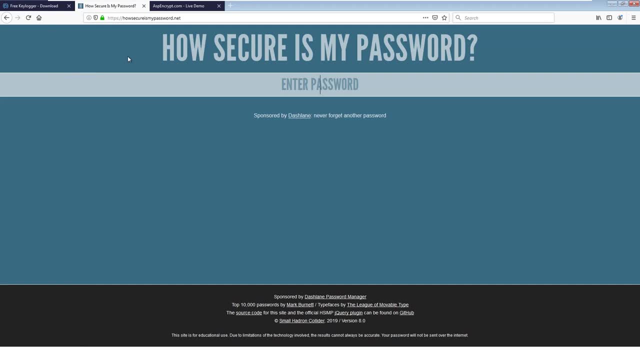 So for the second demo, let's go to this website: how secure my password is, and this will get you a little bit of an understanding of how, how long it would take for a computer to crack the current password that you have. and I don't suggest you actually type in your passwords, but just type in 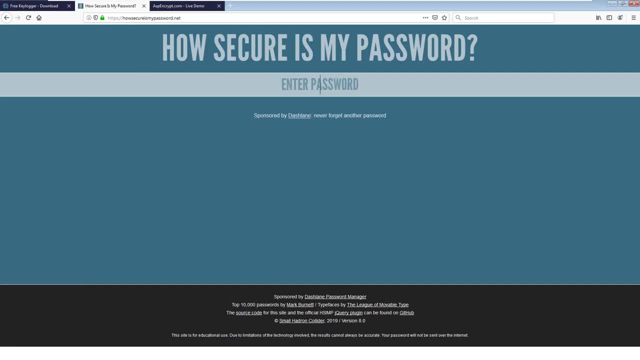 some random words to understand the complexity of a password and how more complex the password, more lengthy the password. it would be difficult for a brute force attack for a computer to conduct right. so here we are, assuming that we are doing a brute force attack. that means that we are going to try each and every combination of the character. 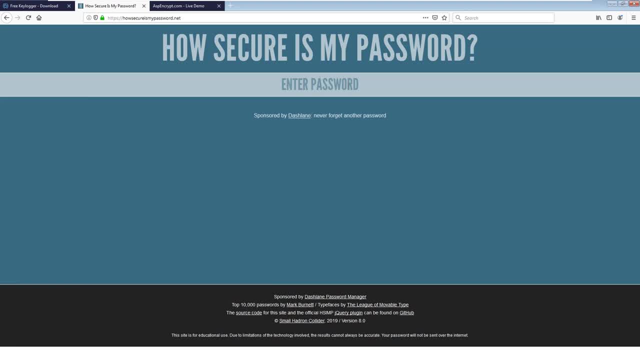 set to crack a password and based on a regular machine, how much time is it going to take for that machine to crack a particular password? when we say a regular machine- machine that an average person can purchase in a laptop or a desktop store, right? so, if I just use the word, 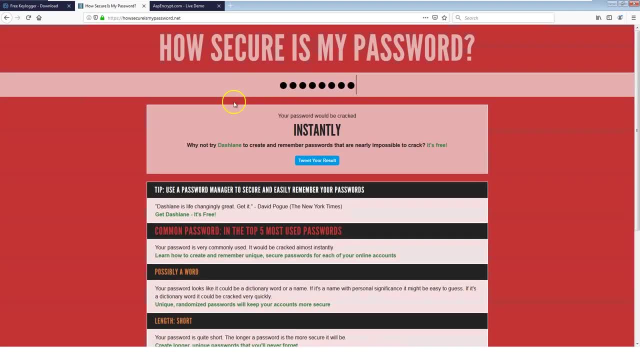 p-a-s-s-w-o-r-d. you can see that it can instantly be cracked because it's a very well known password. if you scroll down, it will also tell you that this is a common password in the top five most used. so people actually use this word password as a password. if I use a variant, let's say I do a p- 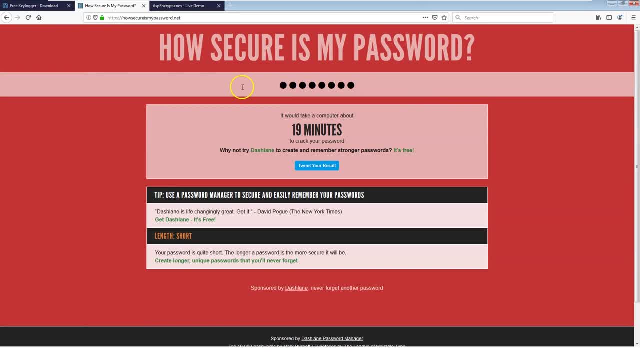 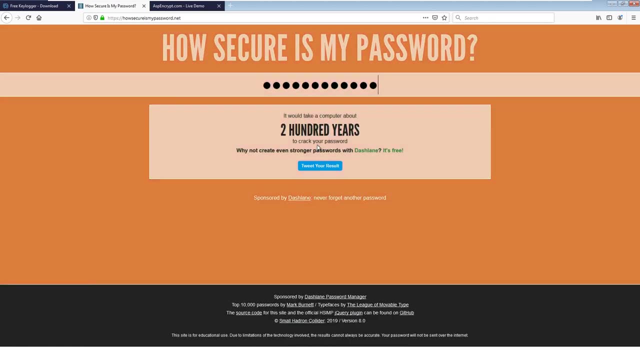 at the rate s-s-w-0-r-d, you will see that if, even if it's a variant, it would take 19 minutes for the computer to crack this password, and if I just add a few numerics, so we have p at the rate s-s-w-0-r-d. if I add one, two, three, four at the end, you can see that, since the password is now, 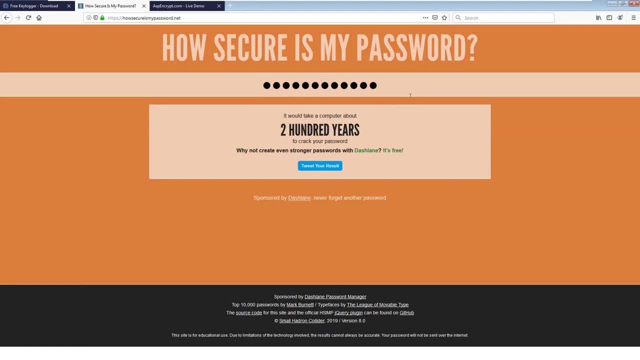 lengthy enough, even if it is not complex, even if it is not randomized, since the length of the password is quite big now, it will still take 200 years for a regular computer to brute force this password. even if I use random words, if the key length or the password length is weak, it's small. 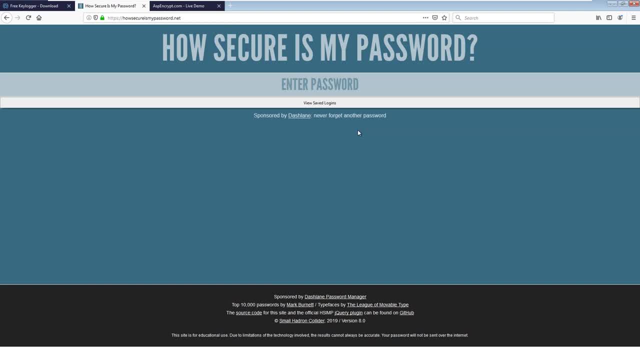 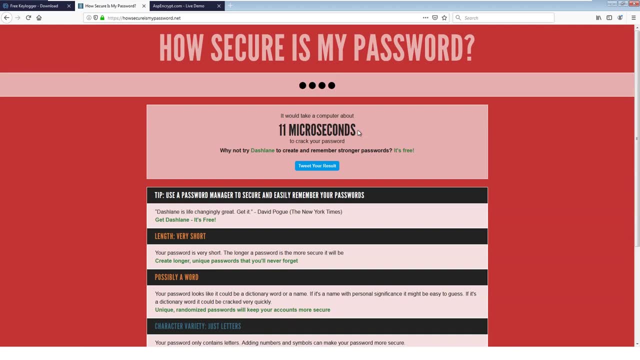 it's less, it would still not be sufficient enough. for example, I'm typing in generic characters b w p. you can see it's 400 nanoseconds, 11 microseconds. b w p, a, f, t w p. so even if I'm typing in random characters right now, all of them are. 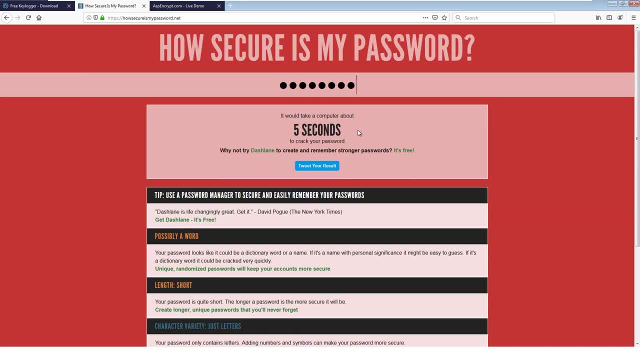 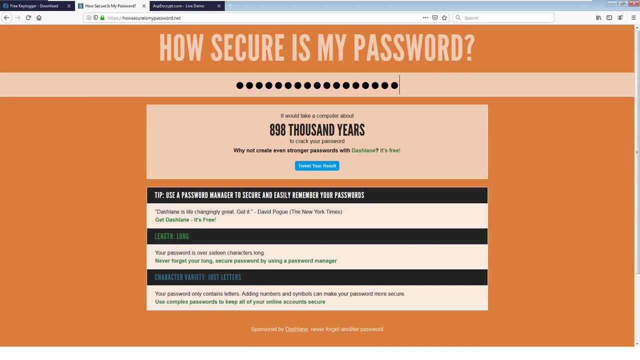 okay and they're easily guessable. so it would still take five seconds for a brute code, brute force attack, to work. but as I keep on typing in random characters and if, as I increase the length of the password, you can see the number of years that it would take is increasing. 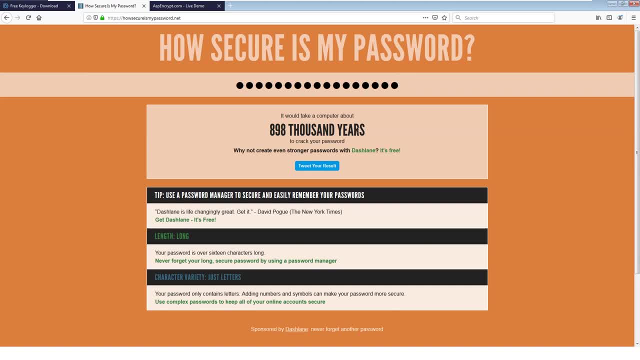 phenomenally, it is now 898 000 years for us to crack this password. I don't even know what I have typed so far, but since the key length is strong, the password is now efficient enough to withstand brute force attacks. right? so that's the reason why I'm typing in random characters, because I'm not. 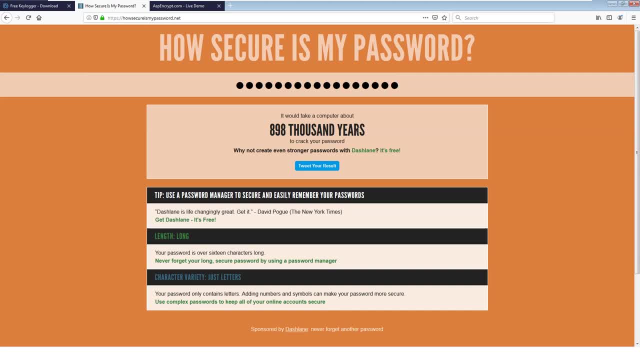 typing in a password. I'm typing in a password because I'm not typing in random characters, right? so this is the reason why- not only randomness, uh, we creating a random password is important. we having number of characters in a password is also very important, so I would suggest to have at. 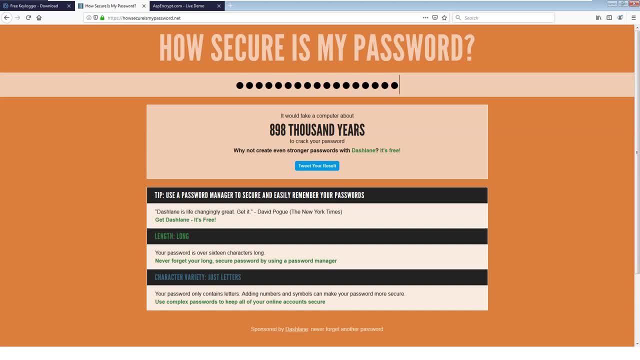 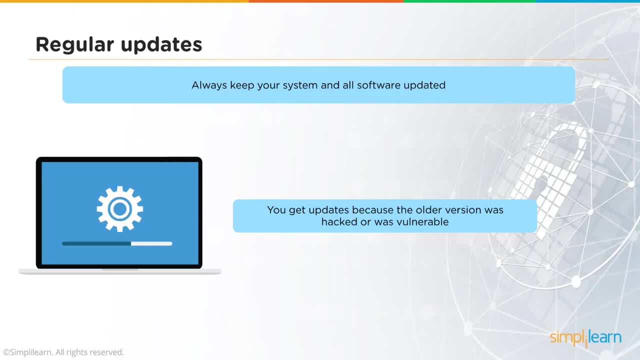 least 12 characters to 18 characters in a password for it to be effective enough against brute force and dictionary based attacks. regular updates for all the softwares is recommended. in fact, if possible, uh, set it up for auto updates if you're not comfortable with that, because it may require. 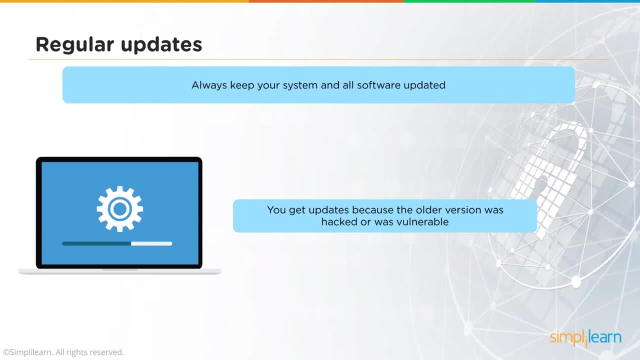 restarts and, uh, it may consume a lot of time. it will need to take a bit more time to create a new of bandwidth in the background, especially if you are doing something that consumes bandwidth. for example, you're on a wipe call and then suddenly something triggers an automatic update. so we don't. 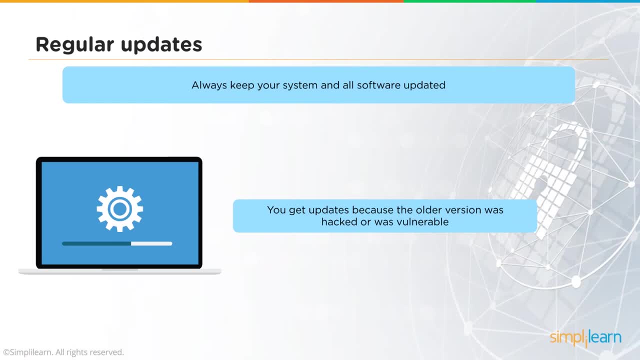 want those scenarios to happen, so you can still keep them on a manual basis, but remember to at least check for updates once in a while. maybe once or twice a week would be recommended. over a period of time you would realize how often the updates of an application are being sent, and then you can. 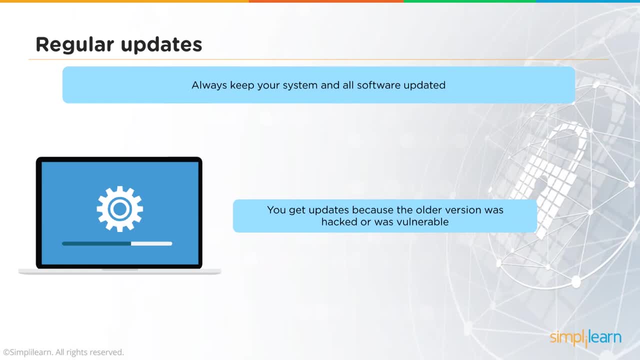 customize and you can then vary your updates or checking for updates as per your feedback that you're getting. so you get updates because the older version was hacked or was vulnerable. some vulnerabilities could be reported by third-party users or some organizations do a vulnerability assessment- penetration test themselves over a period of time, realize there are some flaws. 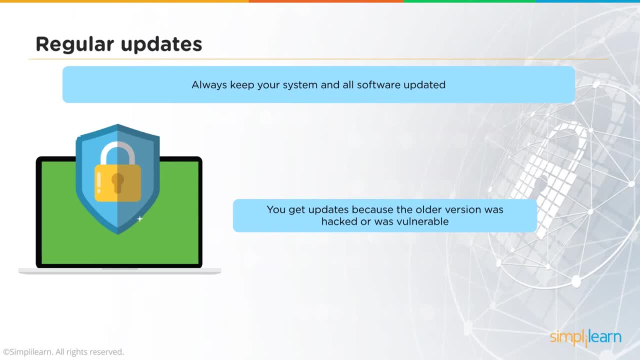 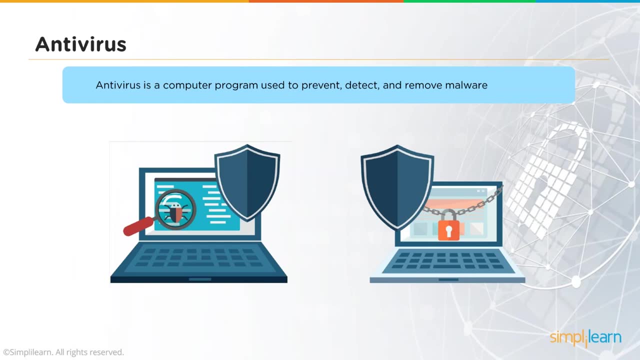 and will create updates and send it across to mitigate vulnerabilities. antiviruses in today's world are a must. you need to keep these antiviruses and again, an antivirus would be the perfect example of updates being installed. almost on a daily basis, you will find new signatures being created for new viruses and worms and malware that has been found. 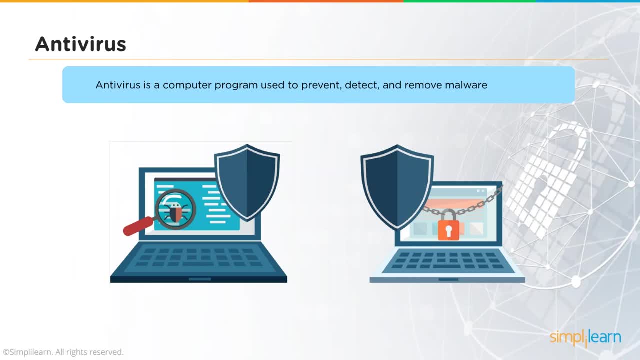 on the internet. so we? it's just not that that we install an antivirus and we forget about it. we have to install the antivirus, we have to keep it updated. there would be updates to the core antivirus that would be released by the organization over a period of time. not only that: your signature. 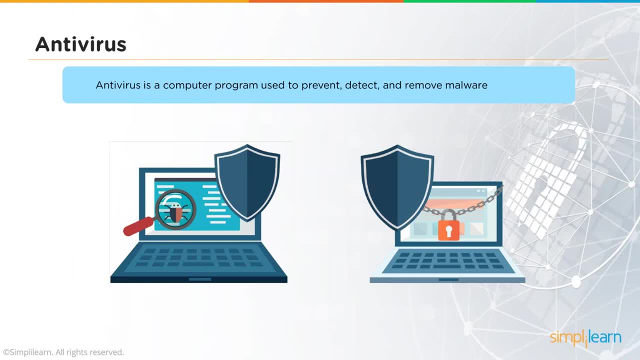 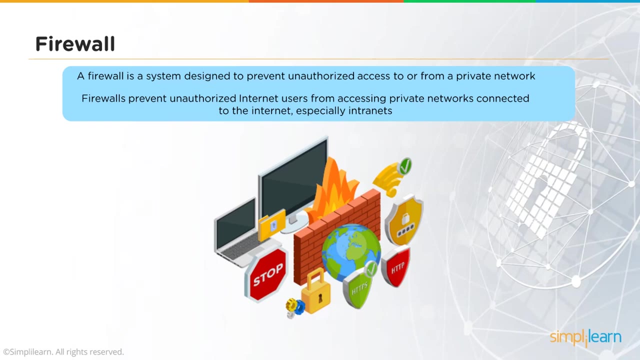 databases would be updated regularly- almost daily- for new, newly identified viruses, worms, Trojans, etc. so installing an antivirus and then keeping it updated is a wanted task. firewalls, as discussed earlier, is a system designed to prevent unauthorized access to or from a private network. now what is authorized and unauthorized is a little bit different as far as firewalls are. 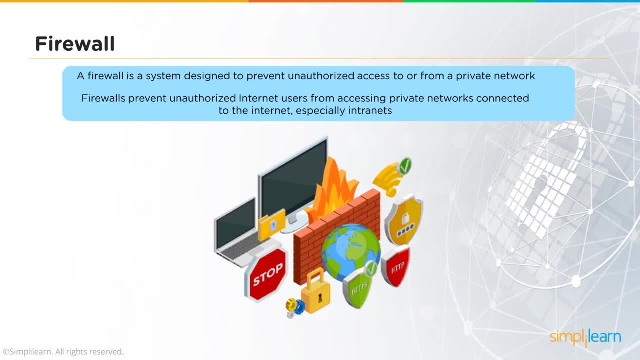 concerned. firewalls will not be looking at users and passwords, but they will be looking at connections, so you can configure a firewall based on ip addresses, port numbers, mac addresses and maybe even a web application firewall with certain scripts that are allowed or disallowed. we'll be discussing firewalls in details later on in a particular video. right now let's just focus on 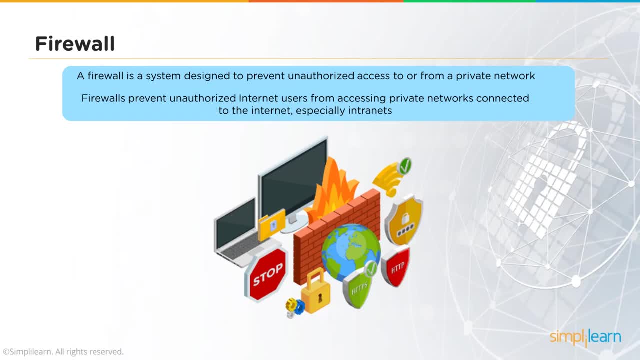 having a good firewall installed and having it properly configured. and this is where the technicality comes in. so you want to allow a particular channel to to be utilized and you want to disallow another particular channel from being utilized, you have to create the specific rules in the firewall. so at the network level itself, if any threat 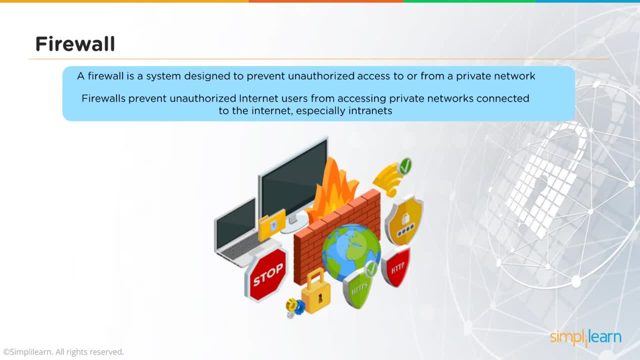 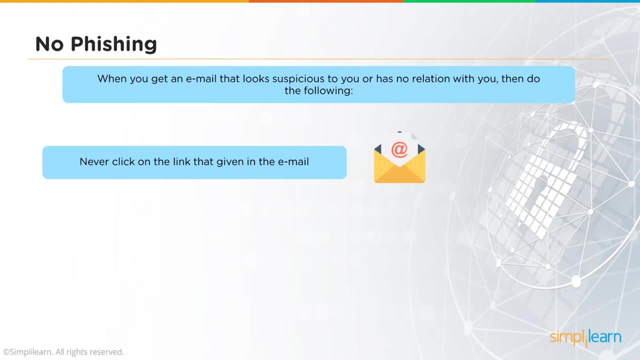 is created, the firewall will try to mitigate it once and for all. phishing: when you get an email that looks suspicious you have or you have to no relation to with, then do the following: never click on that link given in the email, for example, you will get a lot of hyperlinks. maybe you get a. 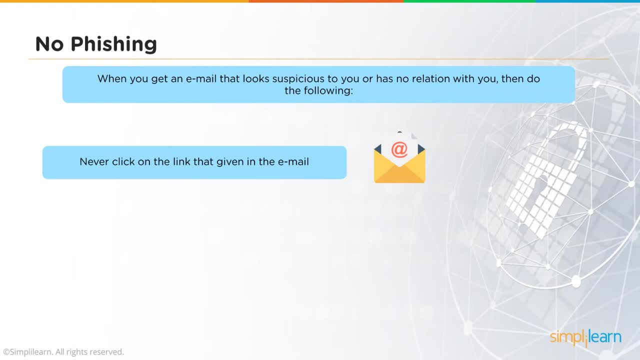 very genuine looking email from facebook saying there has been some unauthorized activity on your account. click here to verify your account, verify the authenticity of that email. do not click on those links. uh, check the header of the email, see where the emails actually come from, and then click. 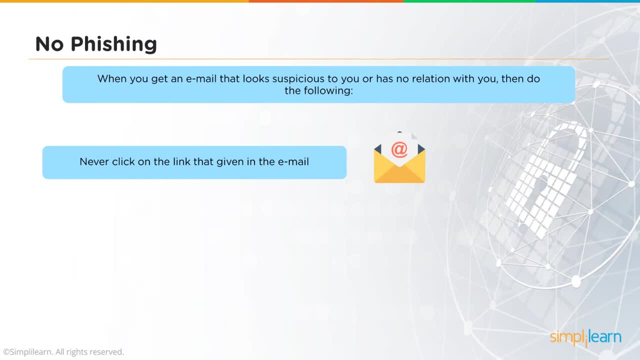 on the link and if yes, that's fine. if not, something is wrong or the best thing is right. click on that link. click on copy link location and paste that hyperlink in a notepad. you will get the underlying path to where that link heads. to verify that the path is correct is actually owned by the. 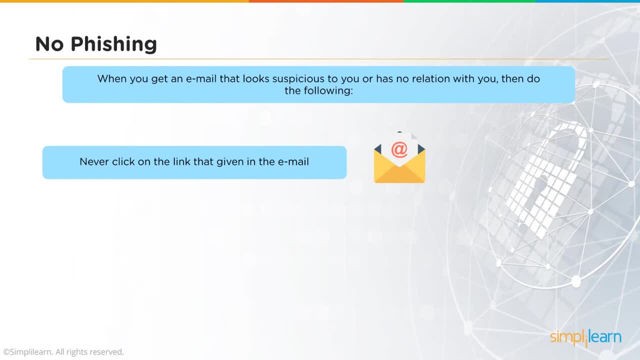 organization who the email is representing. if yes, everything is fine. if not, something is wrong. do not give any personal information or details. if asked, you will see a lot of lottery winning emails coming in asking you for personal information like date of birth, phone numbers. all of these are very important to keep ourselves secure on the internet as well. 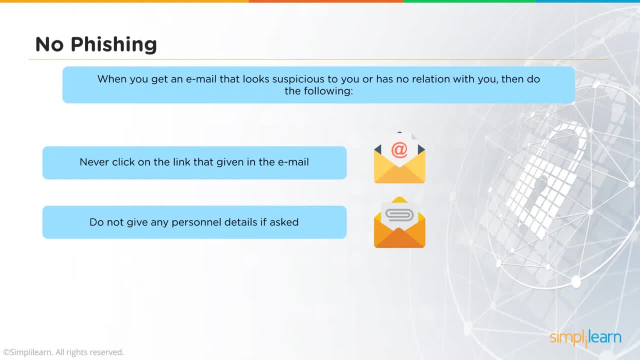 our identities could be leaked out and somebody could then hijack our identity and create a walk for us. so only give out information to trusted people. if you do not trust the email, try to verify the authenticity. if you are unable to verify the authenticity, reply back with a. 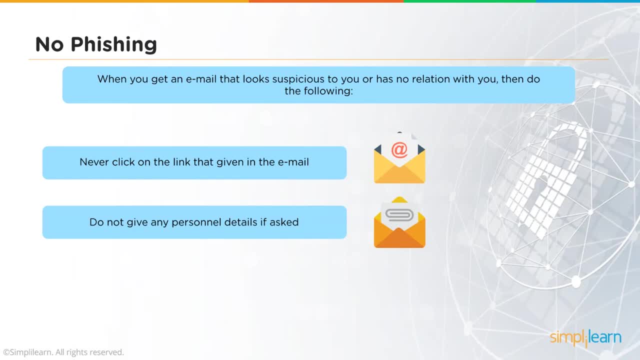 generic questions asking for further information about why you should reveal that information. if it's a genuine email, they would obviously respond with a favourable answer. if it is a um. if it's not a genuine email, you would not get a response. do not open the attached files, so if you're getting attachments from unknown recipients, 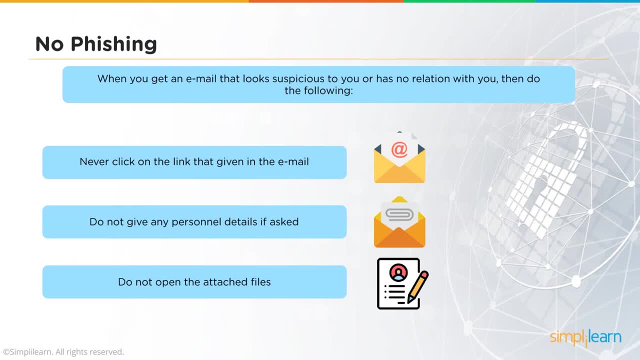 or unknown senders and you're not, you're not able to trust that email. do not open the files, or do not even try to download those files and try to uh look what those files are all about. it could so happen that there would be a virus, worm, trojan in that file and your computer could get infected and 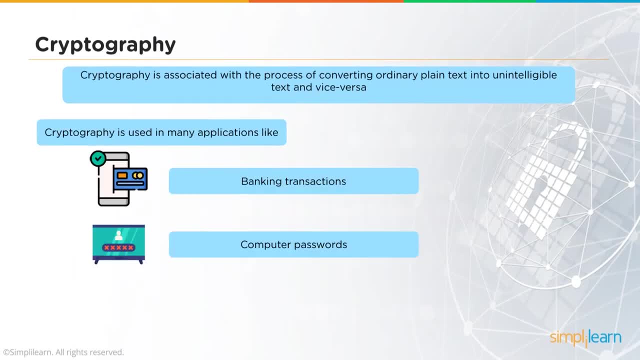 then cryptography, or the encryption process part that we talked about. Encryption is best used to protect our data, the confidentiality part of it. So cryptography is associated with the process of converting ordinary plain text into unintelligible text and vice versa. So when we want to mask data into being unreadable, 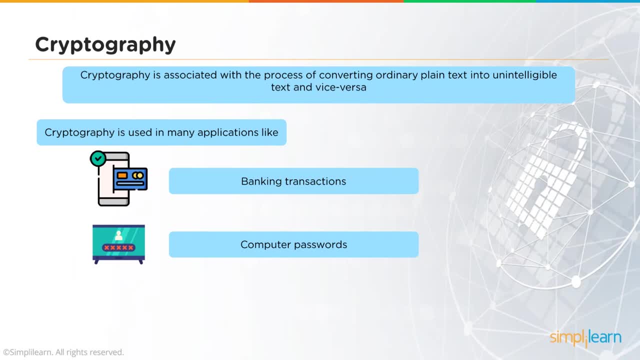 so if somebody hijacks that data, they would still not make sense of it. then use cryptography or encryption. So on a regular basis, your banking transactions will always be encrypted with the highest standards prescribed by PCI DSS. Computer passwords- they would not be. 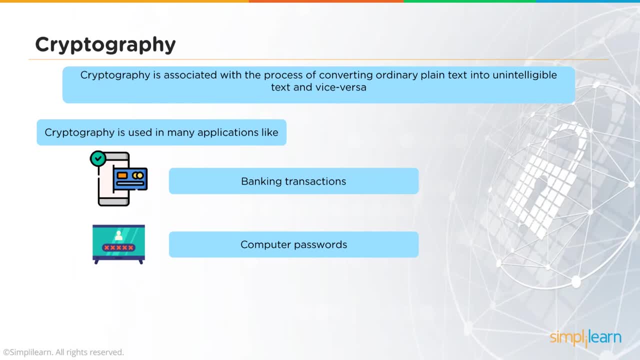 encrypted per se, but cryptography would be used to hash them and store a hash of the actual password in the database rather than storing the clear text, And e-commerce transactions would be encrypted at any point in time. Apart from that, if you want to encrypt your own data or your own, 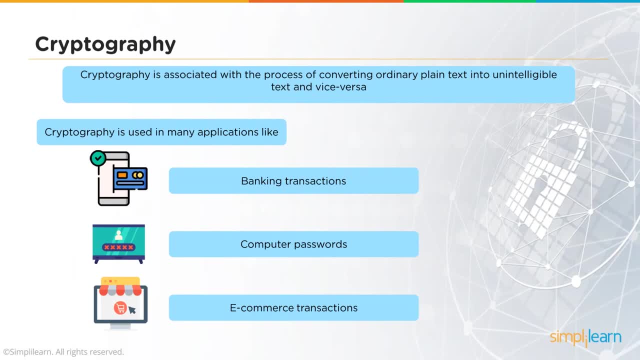 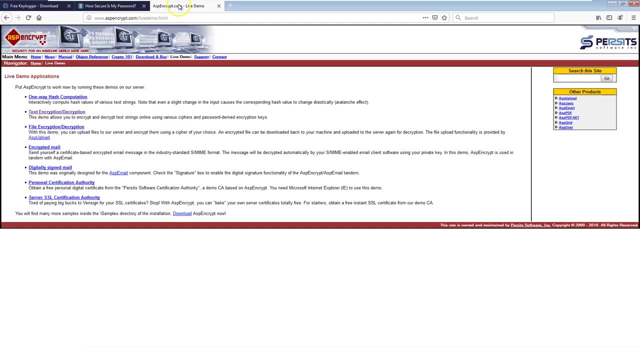 transactions or any other communications that you're making. it's up to you. We'll deal with encryption a little bit later as well, but there are a lot of options out there That will help us encrypt data. So let's move on to the third demo We are going to look at. 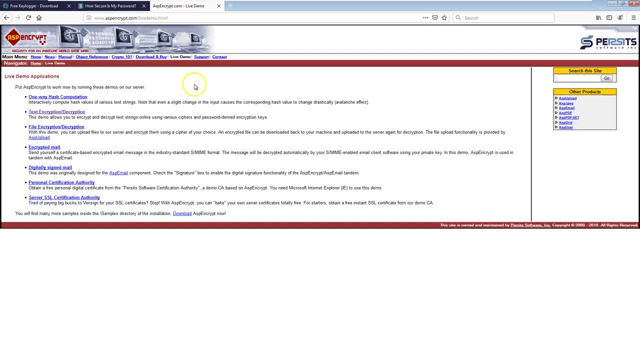 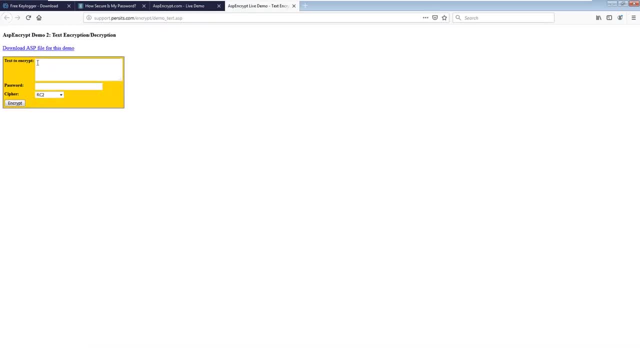 encryption or we're going to look at cryptography, And this is one site which allows us to look at text encryption and decryption. So how does this work? If I click on this link, it will take me to an application which allows me to encrypt a secret message that I can type. So I'm going.